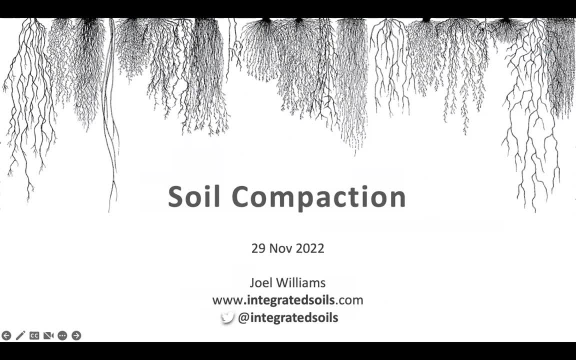 the reality is, if we talk about sore health or sore compaction or sore erosion- as we'll do next week- they are all very interrelated. There's a lot of overlap and common ground between all of these And indeed, when we optimize sore health in a general context, we do also help to alleviate. 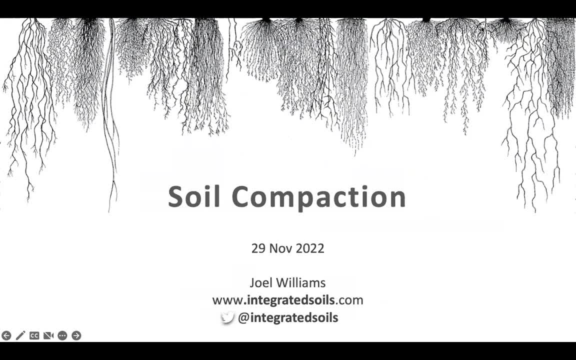 and reduce compaction issues or erosion issues. So there's a lot of overlap here. So some of the themes that we touched on- for those of you maybe that weren't here last week, there will be a little bit of carryover today. So, yeah, you can obviously catch up with that. 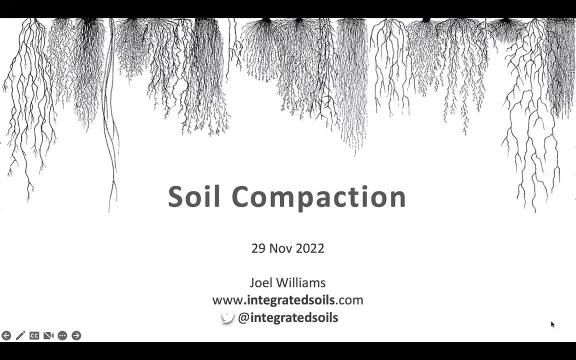 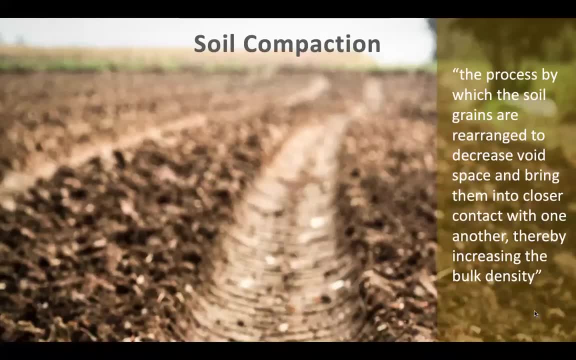 when Kate uploads those to the online. So okay, so let's dive into it. Compaction, Firstly: let's just start by defining what we mean by sore compaction, And really it's just a general process by which the soil grains or the soil particles are rearranged to decrease the 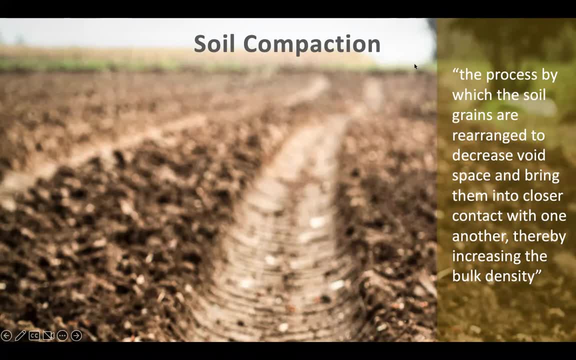 void space and bring them closer together, in closer contact with one Another, Thereby ultimately increase the bulk density. So, as it explains, really, it's really just about compressing all of the soil particles together, bringing them closer together. and when we compress the soil, 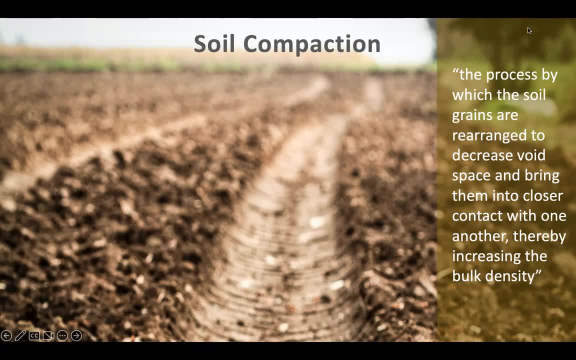 particles, bringing them closer together to round the tidal з instances. That means we're earnestly mismanagement and bi accelerating both types of composition, including different types, And if we stop together, of course, what we are really losing out on in that, through that process, is the poor space. 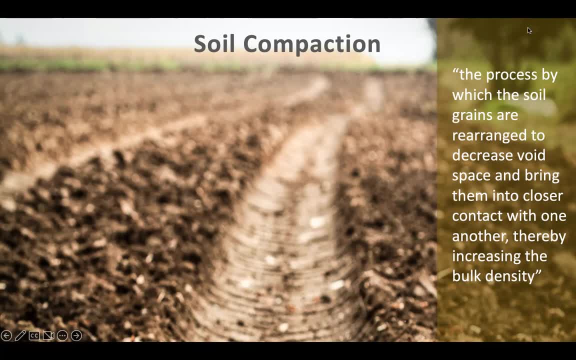 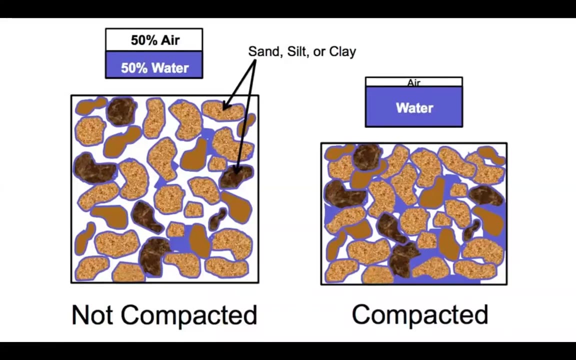 the space in between the particles is what is the key thing that we are losing through compaction, by compressing all of the particle, the soil particles, together. so some visuals to kind of expand on this or just clarify this. so here we have a nice open, structured soil where we have 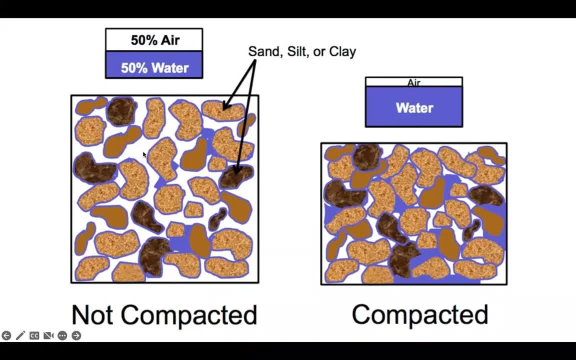 lots of space for air and then space for water to to kind of stick to those soil particles. the water will always adhere, much closer attracted to the soil particles that will adhere to those, creating then the air space in between, the porosity space in between and over on the right. 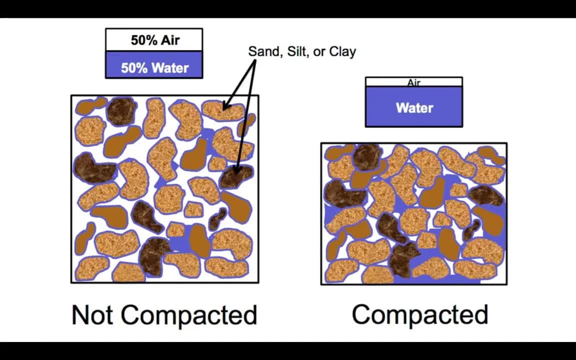 hand side. as you see, when we then compress the soil particles together, we have a lot of space in between the porosity space in between and over on the right hand side. as you see, when we press that, we're pretty much losing air space and that means as a percentage, that the water 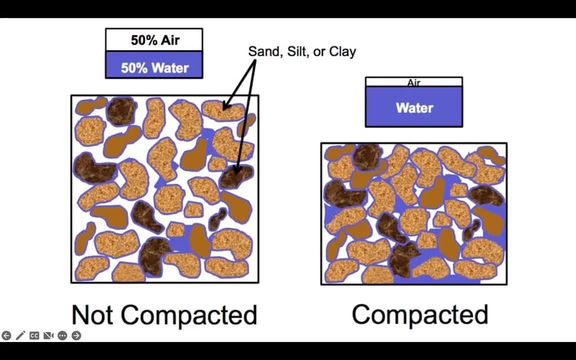 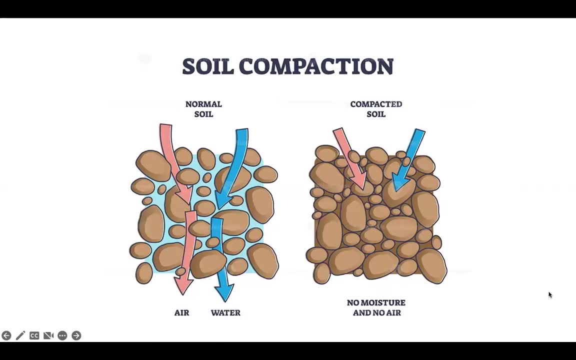 really starts to fill up more of those gaps. so, relatively speaking, as a percentage, the water takes up more, thereby leading to waterlogged conditions and lack of air, lack of gas. exchange some other again i'm just going to show. throw a few different images of the same thing really, but 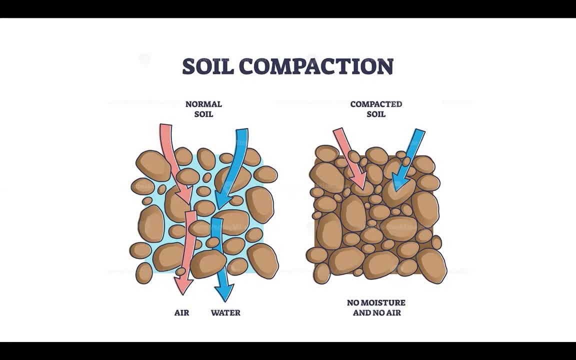 just nice visual cues to kind of explain this. some other again. i'm just going to show, throw a few different images of the same thing really, but i think i what i really like about this image, of course, is um, on the left hand side. there we have this good structured soil where 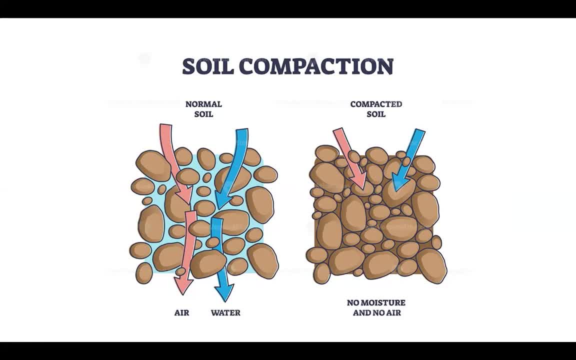 not just. also water can get in, so for example, rainfall can penetrate, infiltrate down into the soil and percolate down through that soil profile. but also we have space, again that pore space for air, for oxygen to move in. but oxygen is really important to feed the organisms down in the soil. 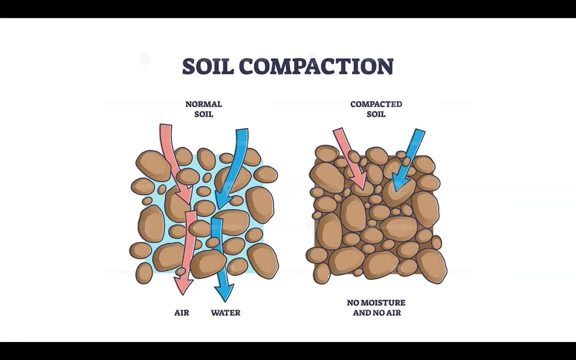 all the microorganisms and other um, insects and worms, etc. but the pore space there is not just important for air to come in, it's also important for carbon dioxide to come out, because all of the life in the soil, or the biology they are, as they grow and do their thing in the soil, they are respiring, they are releasing some co2, just like. 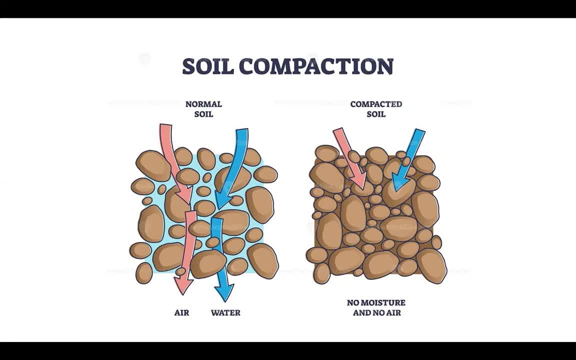 we do. we breathe in oxygen and release co2. they do the same and that's co2 that comes out of the soil. is actually very important for it to leave the soil where it can be taken up by the plant and then recirculated back in. 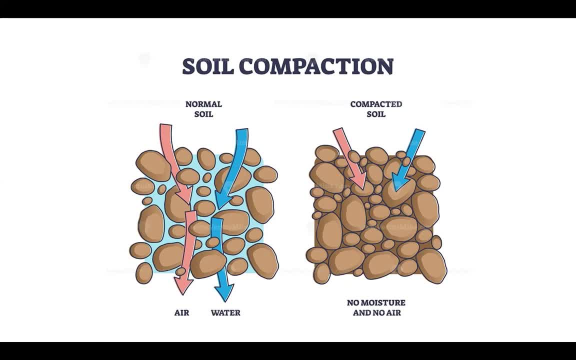 recycled back in for photosynthesis. So indeed, good, well-structured soil, uncompacted soil, is really important for gaseous exchange, for oxygen to come in and CO2 to come out, as well as then water infiltration and water movement around the soil. 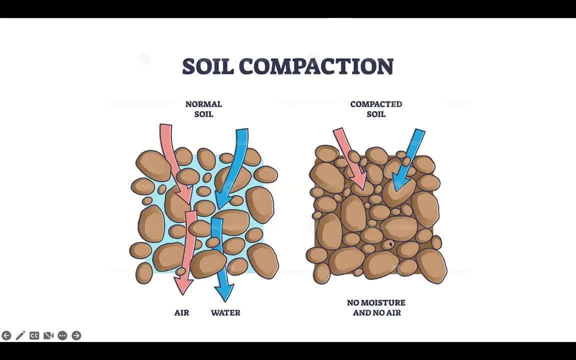 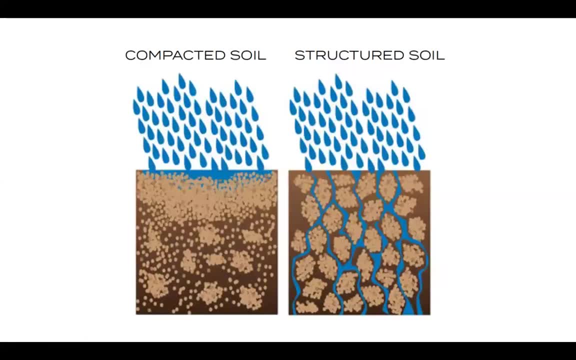 So, of course, once we have compacted soil and we tighten those particles up, we just have no space for that water or air and gas exchange. And another example: here again, we can see well-structured soil where, when we have- and this is really leading to next week's conversation- 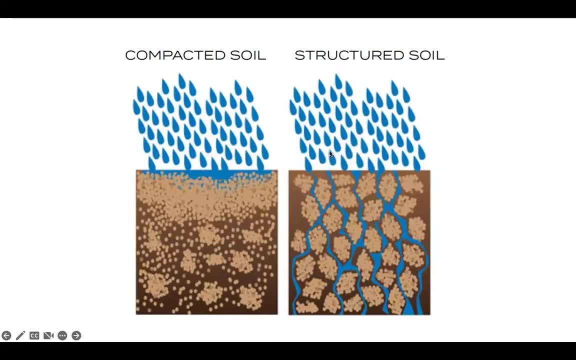 where we have a rainfall event, in a well-structured soil, that water, because of the pore space, will be able to infiltrate and penetrate, as we just mentioned. However, when we see when we have compacted soils, that is then where that soil begins to accumulate. 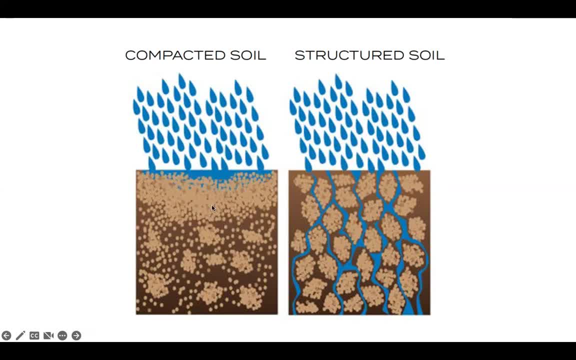 on the surface and does not move down, We don't see vertical movement of that water down the profile. And so when we don't have good water infiltration and water sits on the surface like this during high intensity, heavy rainfall events, then the water of course has nowhere to go. 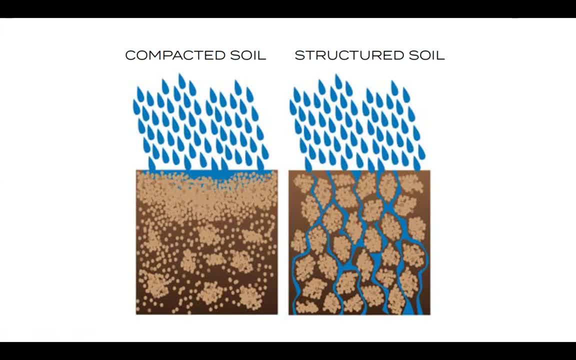 nowhere to go down. It has to go across And that's where we start the process of soil erosion. So we'll elaborate on that next week, but clearly these two things are very tightly intertwined. Once we have compact soil, you are running the risk of soil erosion. 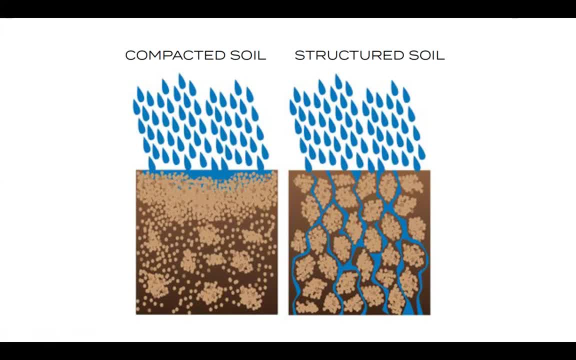 And at least compaction is not ideal, of course, but at least it is reversible. We can work on that, which we'll talk about now for the rest of the presentation, But soil erosion, however, is not really a reversible process. 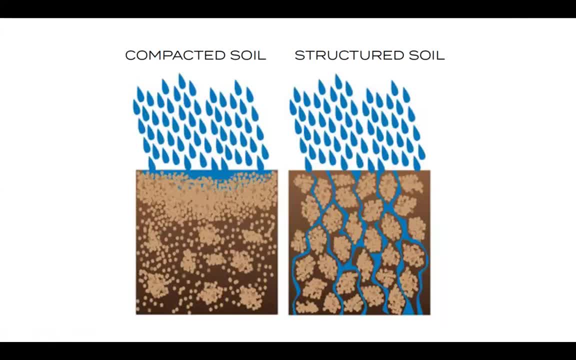 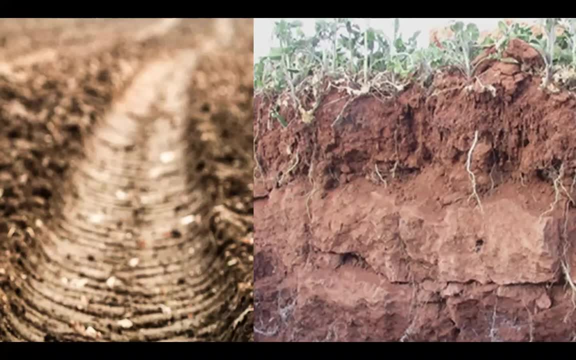 If that's once that's washed away and leaves the farm gate, anyway, that precious resource is gone. Okay, so let's have a look at some photos. then Compaction: again, we're just compressing particles or particles together, And some of that compaction can be on the surface. 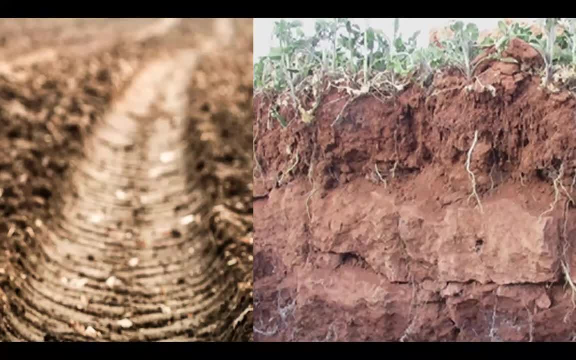 As you can see, on the left we have a lot of surface compaction through that tire track And on the right-hand side, I would say actually very common problem and a little bit more insidious, a little bit more difficult to diagnose. 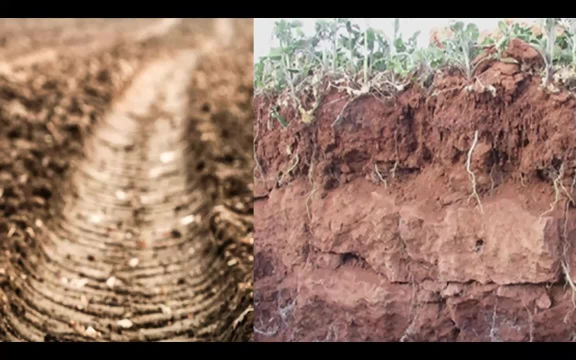 perhaps going a little bit more unseen commonly is more of some subsoil or below surface compaction And you can see this layer here through the middle where we have very tight soil. We're seeing very smooth soil. We have very nice, very smooth surfaces. 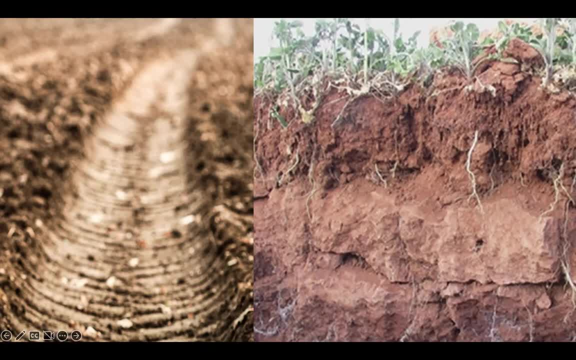 Up here we have a much better structure. We have some roots and some texture. It's not so flat and smooth. We have kind of a textural kind of dimension there to that layer. So we have three-dimensional kind of particles with space, with depth, that kind of thing. 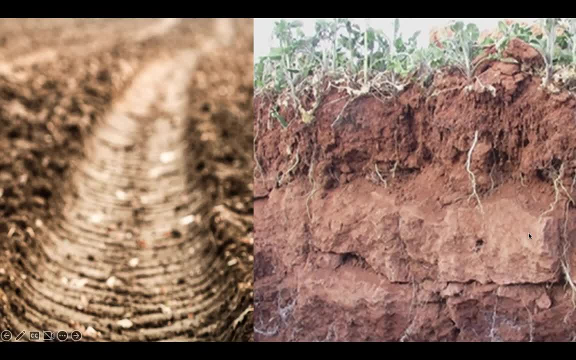 Whereas at the bottom there, we have this distinct kind of flat, smooth layer, um, and, of course, uh yeah, unless you're out there digging and um, having a look in your soil, you, you, this kind of subsoil compaction may go undiagnosed for some time, but, as you can, 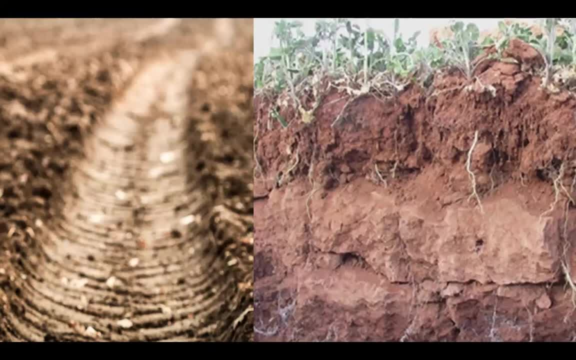 obviously see and imagine. you know, root growth is, um is uh, limited here. the roots can grow through the soil surface, but once they hit that compaction layer it becomes very difficult for roots to get through. and i mean roots. i'll talk about roots later. roots are amazing things and 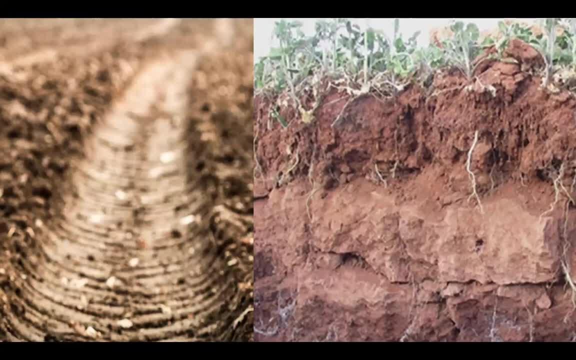 indeed, they can get through lots of very difficult and challenging circumstances. but, um, but of course they, they do that very slowly, it's, uh, they don't do it very effectively. um, you're not going to have good. therefore, you know, without good root penetration, you're not going to have good. 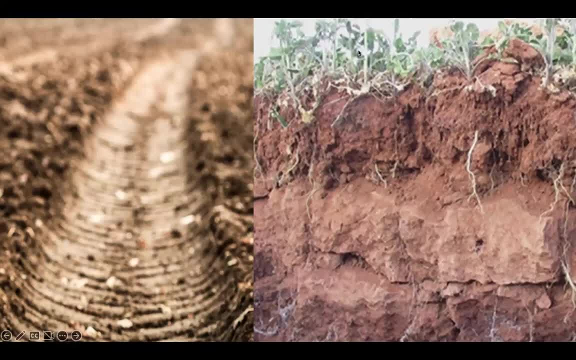 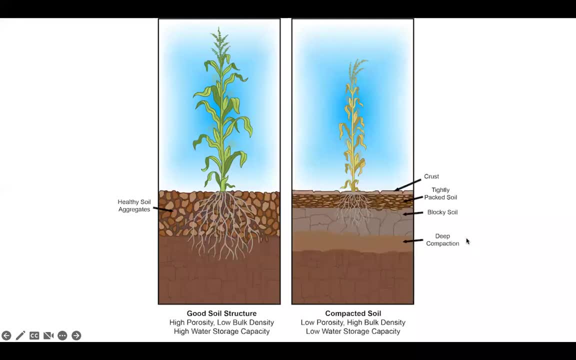 moisture access, nutrient access. therefore, you're not going to have good production up top. so, um, it's uh. roots can overcome such challenges, but, um, it's a difficult and slow process, and we'll talk about at the end strategies to alleviate compaction. so, again, just some nice. 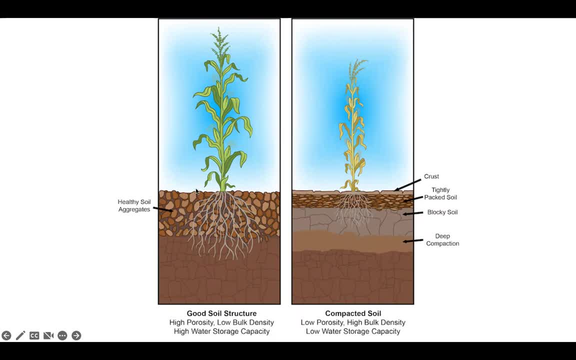 visual cues. you know, when we have good soil structure, good aggregates, good space between pore space, the roots can just move through those spaces, push particles or particles away and penetrate those roots. when we have these compacted layers like kind of what we just saw, especially that here's that kind of what they call blocky soil. 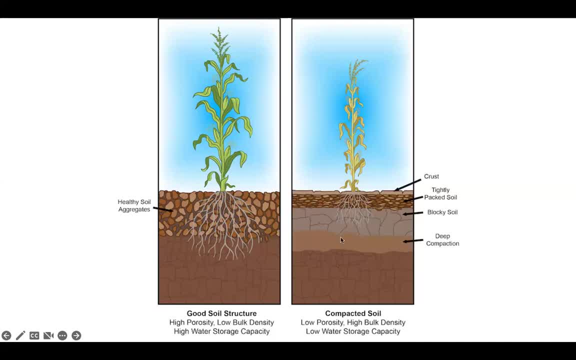 these very brick-like smooth structures and even specifically, very tight compact layers. we can often have these often called a hard pan or very just, very thin layers, but very tightly compressed, often right at the machinery level where maybe historically soils were worked or cultivated, for example, and we'll often see these compact layers kind of right beneath, uh, right underneath. 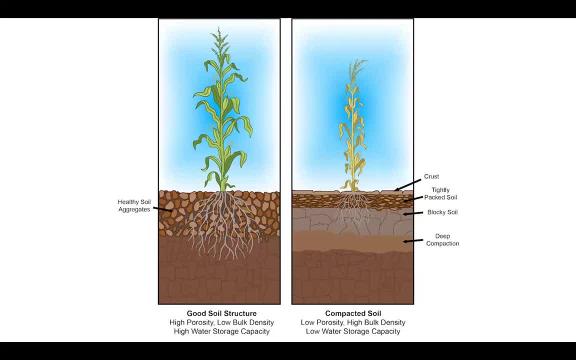 the layer or the depth of soil cultivation. so, um, you know, once we get these kind of especially the subsoil type compaction, yeah, the roots they just they struggle to grow through there and consequently they can't access moisture and nutrients and therefore productivity um will decline and will. 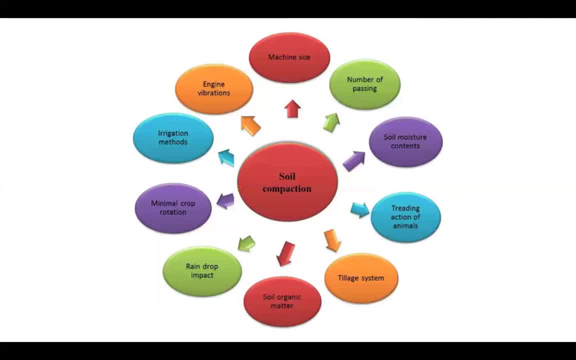 suffer accordingly um due to, due to that type soil. so let's have a consider of some of the causes, the kind of um on the underlying causes of compaction. and of course machinery is a big one. the size of machinery, the number of passing passes that we make with the machinery, even engine vibrations can contribute to to this. 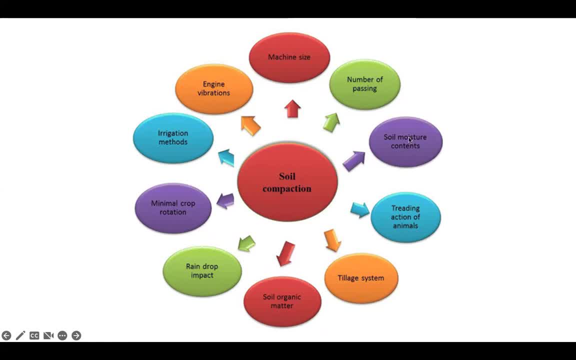 i'm going to come back and talk about soil moisture. this is actually a really important one, and arguably one of the most critical aspects to this conversation about soil compaction is soil moisture, and usually machinery or livestock action on wet soils is the biggest problem. so, of course, overgrazing or 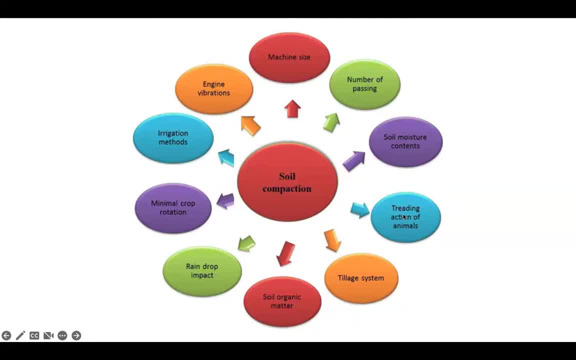 compaction from the livestock is a big factor here. it can be a big factor again. it's all in the management, but we'll come back to that. tillage, excess tillage over cultivations are definitely a problem. low soil, organic matter- we will talk in depth of this. even raindrops- the impact of raindrops- can certainly contribute to. 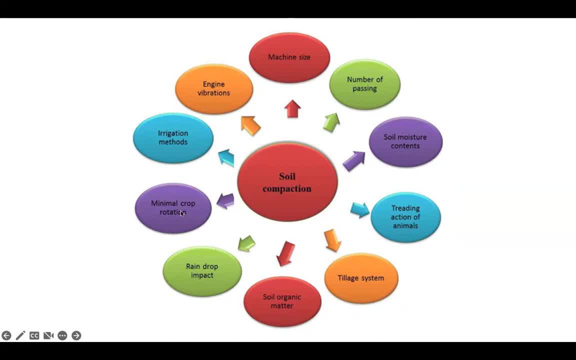 the problem? core crop rotations and um monocultural production systems, lack of agro biodiversity, lack of rotations, lack of diversity. these things are all factors, and even irrigation methods, if we you know, when we think about irrigation- or rainfall, for that matter too, but also irrigation, once we apply a lot of water to the soil- the water itself weighs a lot, you know, and if that particularly, 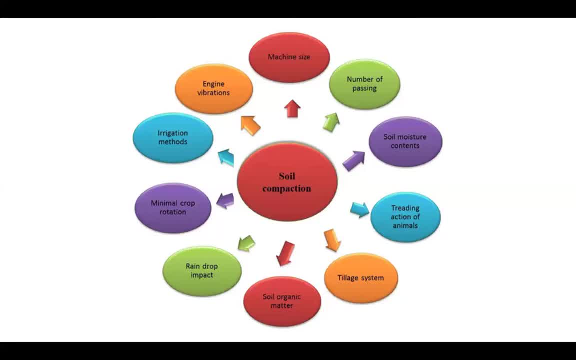 with the rainfall event, if that water doesn't start to infiltrate down through the soil, like those photos we saw, images we saw earlier, if that water is not moving down into the soil and it starts to sit and collect on the top, well, the weight of that water you know? an inch of water. 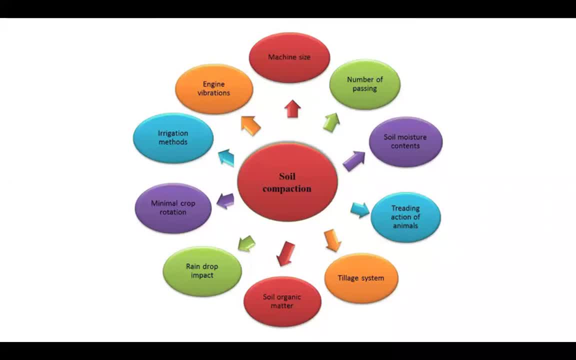 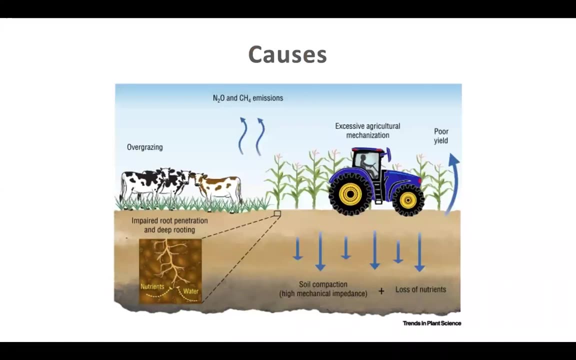 over a hectare or so is, you know we're talking huge tons tonnage of water and so the, the weight of that as it sits on the surface really can also begin to um, compress the, the soil underneath and really the- there's no doubt about it- really the two primary causes of most concern and most 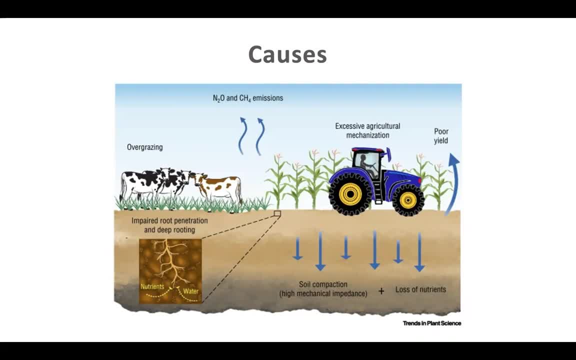 relevance in agriculture generally. it really is machinery and livestock, and it's not to say that either of those two, by default, are therefore um. the problem, necessarily, the whole problem, it's how we use these tools, it's how we um, how we manage livestock, how we track the settings or 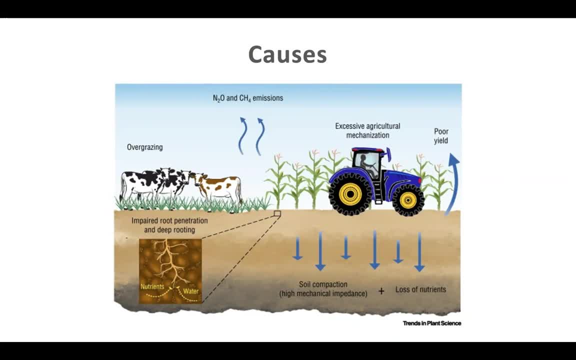 um, as i say, the number of passes in that country, how we use machinery, that that um is typically the kind of the big problem, but but really for sure these are the two that are the primary ones to be concerned of. so really trying to min limit machinery weight and number of passes, um and 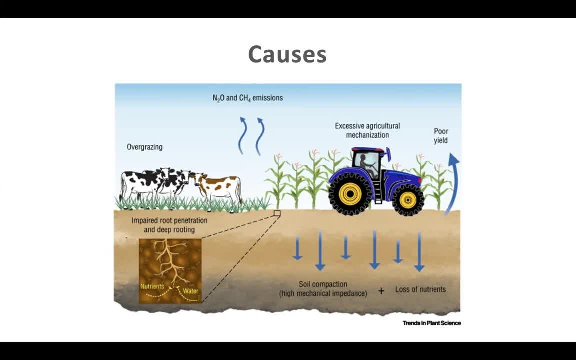 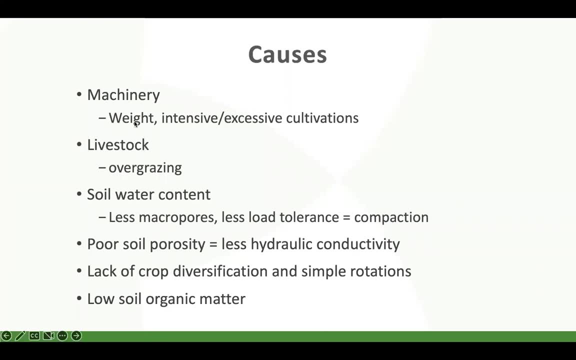 certainly trying to limit over grazing and um from livestock is is two of your key key strategies. so, um, uh, really be on kind of those two um, which are two really key ones. um, it's this point about soil water. when we have waterlogged soil or wet soil- excellent, like good wet soils- excess water in soils, what that? 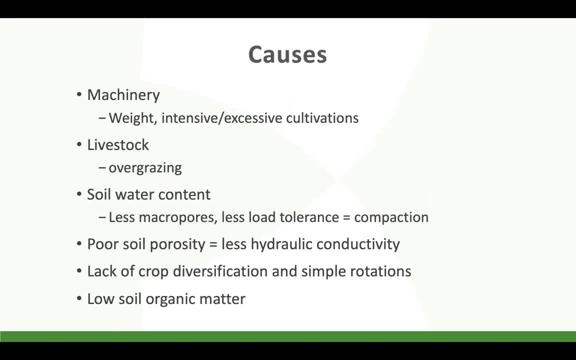 water ultimately does is fill up all the pores, um, those that pore space that we showed earlier, particularly, it's the macro pores. and once you fill the macro pores, what those pores, that this is the space between the particles, what those pores really do, that they, they enable the soil to behave a little like a sponge, you know. 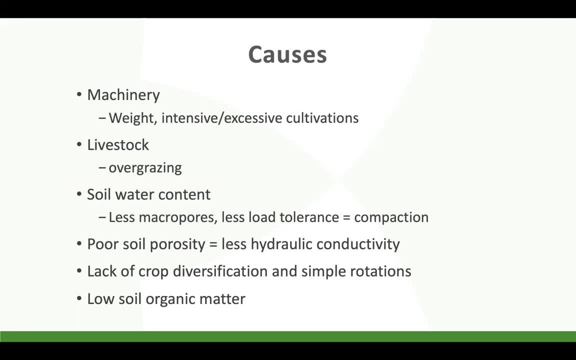 they create the pore space, that in which the soil can compact, can, can tighten and rebound and reflex, and that's really what pore space helps to do by simply having space between the particles. so when we then have compact soils and therefore more water, filling up those pore spaces ultimately, 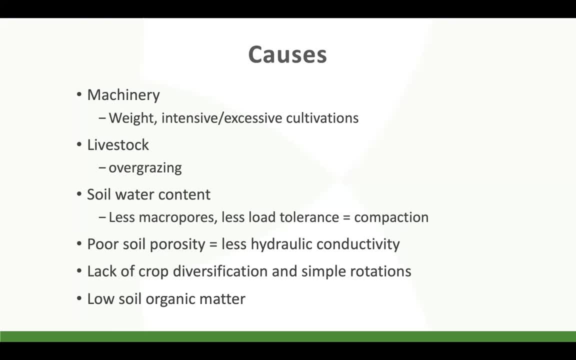 that really means that the Soil has less tolerance to load and that load could be the machinery load that we just talked about, or the livestock load, the weight of the livestock or the hoofs, etc. So they have less tolerance to the load, to that weight or that load. when we have less of those macropores and especially when those macropores are wet, are full of water. 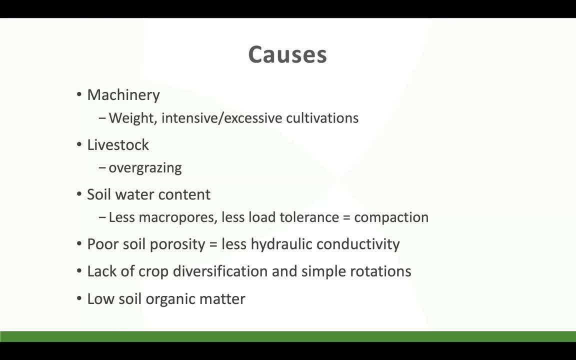 That's really your key driver. cause of compaction is this: wet soils, and then the machinery and the livestock on the wet soil is then what has become so damaging. So really it's about poor soil porosity and when we have a lack of pores, not just numbers of pores or poor area, but also poor connectivity- how well those pores are connected. 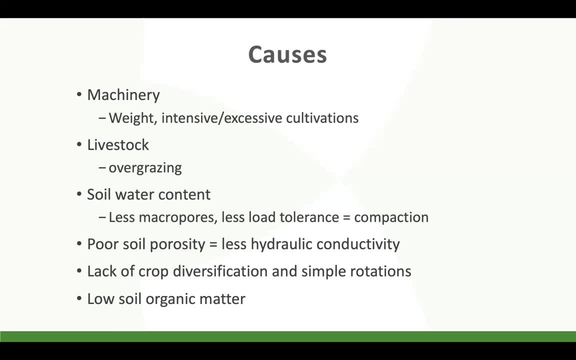 This basically means we have less hydraulic economy, We have less conductivity or less water conductivity, less water movement through the soil. The water needs those pore spaces to move, be that infiltrate, be that percolate down or even just move throughout the soil to move nutrients around. 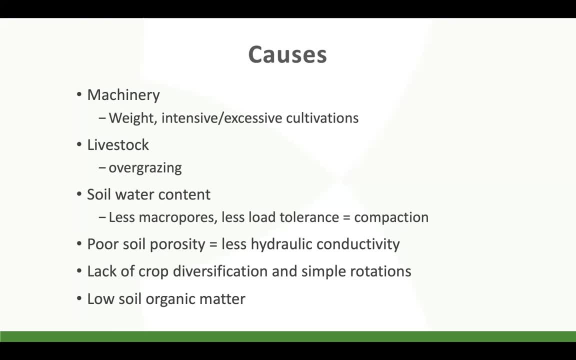 We see less water movement, less water relations, and this is going to be central to the problem, And really one of the big causes of that, as I touched on there earlier, is this lack of crop diversification, simple rotations, monocultures. 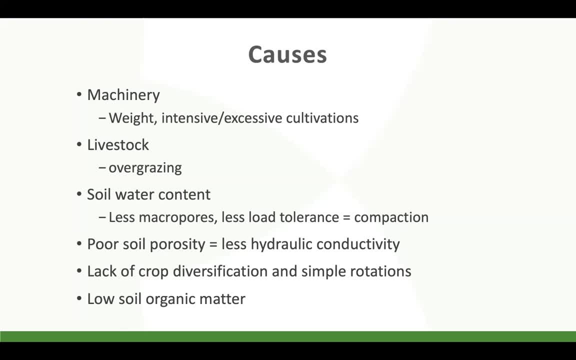 There's a lot of problems with that. There's a lot of problems with that We've kind of transitioned towards. in a lot of modern agriculture It is more diversity of plants, of plant roots, across space, across time that is so central in preventing this problem of soil compaction in the first place. 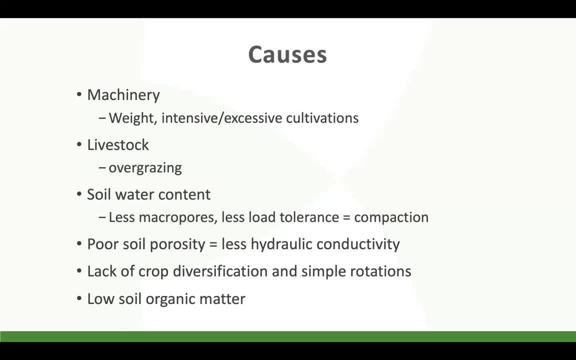 So, as we've kind of really intensified agriculture and lost some of our diversity, this has also been a factor. And then low soil organic, And this is a vicious cycle. I'm going to talk about soil organic matter later, but soils that are low in organic matter are more prone to compaction. 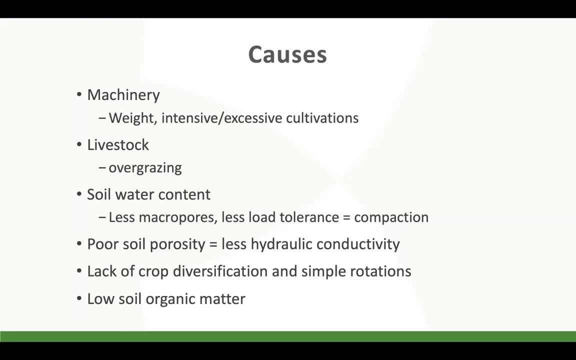 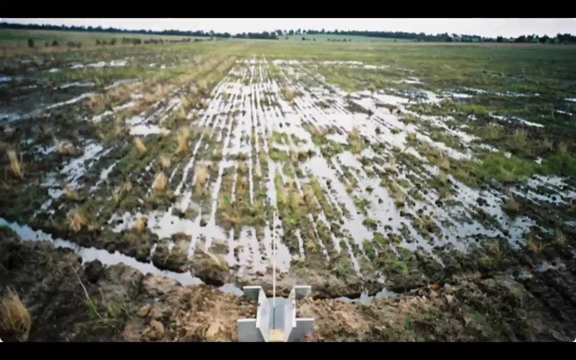 And also it's harder to build soil organic matter in soils that are compact. So we have this kind of vicious cycle there. But definitely if we can build soil organic matter, which I'll talk about, then this helps significantly And really the critical message about soil compact. 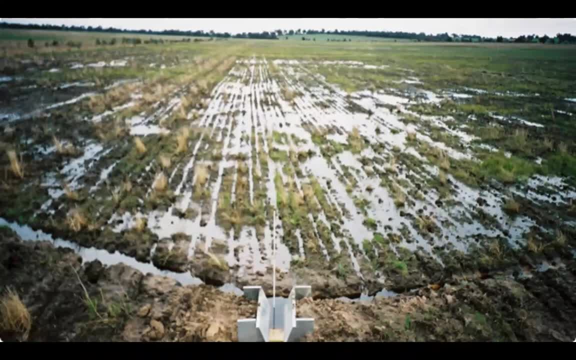 And it's just if the soil is wet, just to keep off it. from a machinery point of view, from a livestock point of view, it's the water logging is not great, of course, and the weight of that water itself, But it is when we go on there and with machinery, with cultivations or with animals, that is then what's really doing the damage. 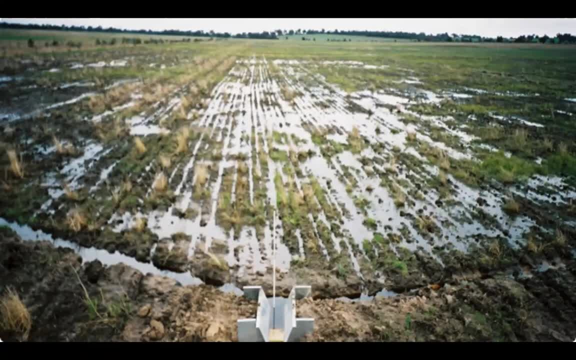 The water logging sets it up And The the animals or the machinery, just you know, finishes the job. So the key take home message, I think, is: just if the soil is wet and not just water log, OK, this is an extreme example of water logging. 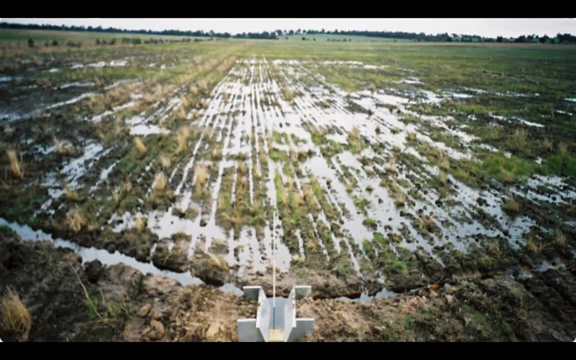 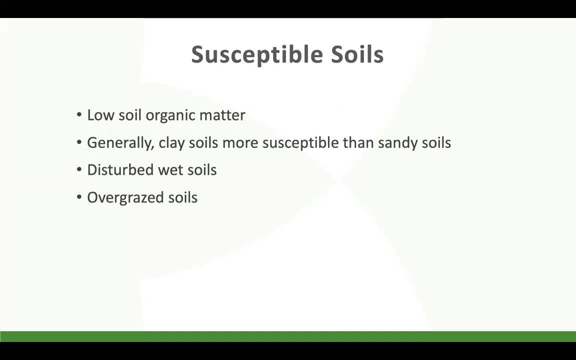 But if the soil is just wet- too wet for working, et cetera- then just keep off it, because you're doing a lot more damage than than good. So there are soils that are maybe a bit more susceptible, or conditions that rise to greater susceptibility. 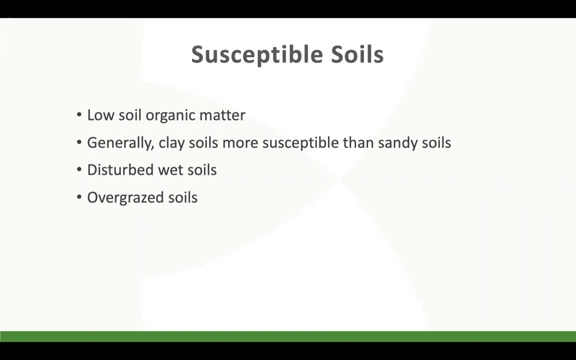 And again, low organic matter. So we're going to come back to this. generally, clay soils are more compactable than sandia soils just because clay soils are smaller particles, finer particles, that they can compact more tightly together, where sandia, lighter soils are a bit more coarse, bigger coarse particles. 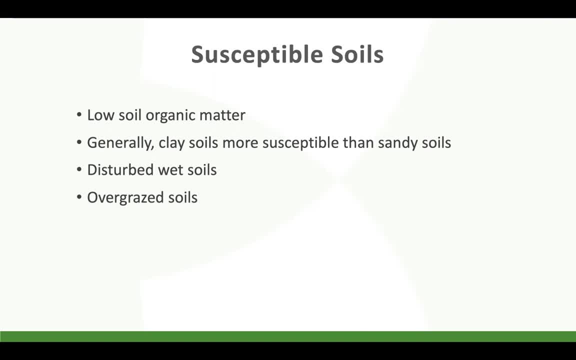 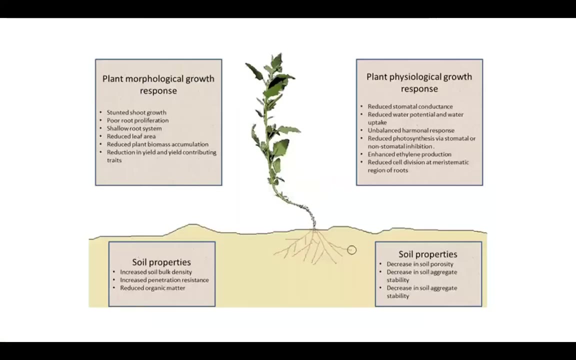 So by default, there's always going to be a bit more airspace between them. Again, those disturbed wet soils, as I've mentioned, and the overgrazed soil, So any any Soils of these kind of patterns- you're particularly vulnerable and prone to to compaction issues. 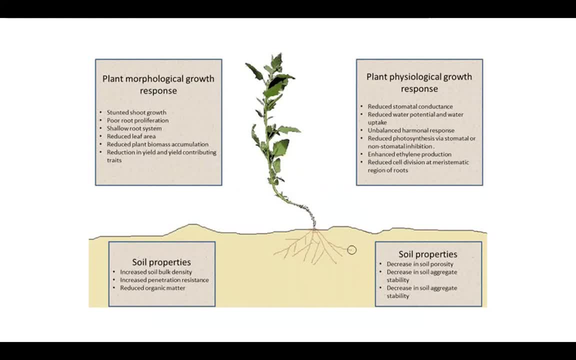 So what are some of the negatives? the problems that we associate with compact soils, And there's a lot of problems for the soil itself, the soil properties, but also for plant growth and plant production. So, for example, obviously with a tight soil we're going to see less, less biomass growth. 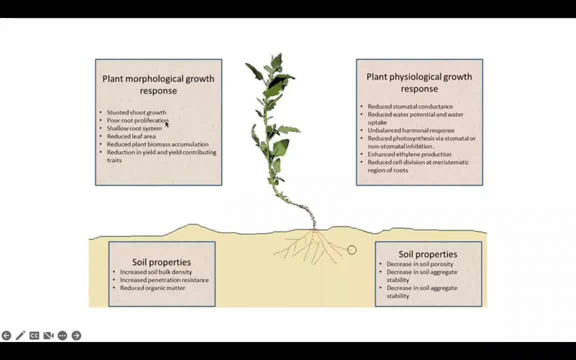 Because we have poor root proliferation and those roots are there to get moisture and nutrients to then drive above ground growth. So we're going to have stunts of growth, poor roots, shallow root system, reduced leaf area, reduced plant biomass And, of course, ultimately this is going to mean less yield for the plant. 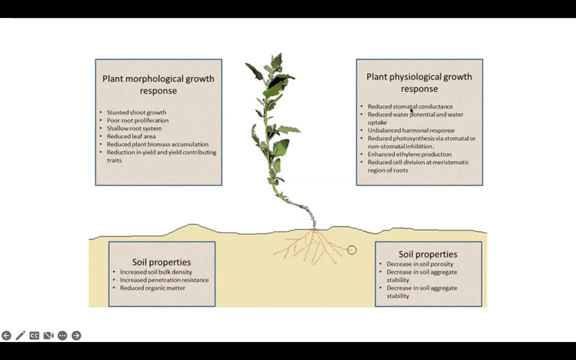 But beyond that also, we have things like reduced stomata conductance, So that basically means poorer photosynthesis. We're not going to have good opening and closing of the stomata to conserve water or to breathe in carbon dioxide. reduce water uptake in the plant, water pressure of the plant, unbalanced hormonal response, reduced photosynthesis, as I mentioned. enhanced ethylene production. 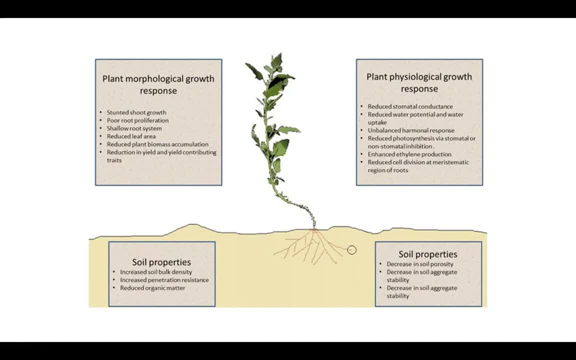 This can be also a stress-related response and ethylene can contribute to cell senescence. So just declines in growth and productivity and reductions in cell division, which is how plant root and shoot tips grow at the very tips is, through cell division, particularly problematic in the root areas. 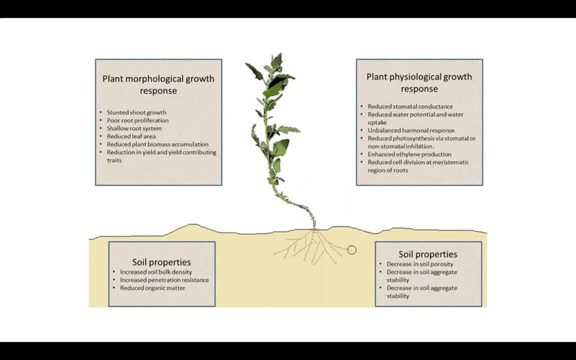 But for soils, then it's this increase. the compression means increases in bulk density, which really just means to increase penetration resistance. So tight soils that roots cannot penetrate is obviously the big problem. This leads to less organic matter- I'll come back to this- and decreases in soil porosity, as we touched on decreases in soil aggregates, aggregate stability and again aggregate stability. this is one that will overlap to next week when we talk about erosion. 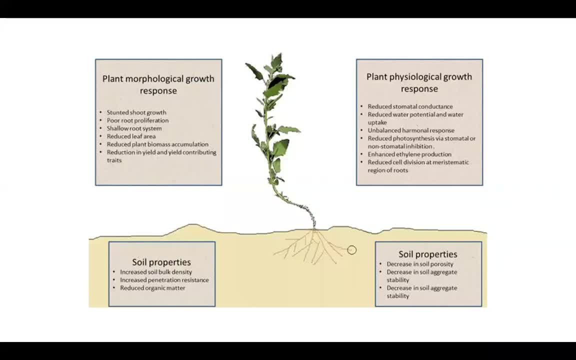 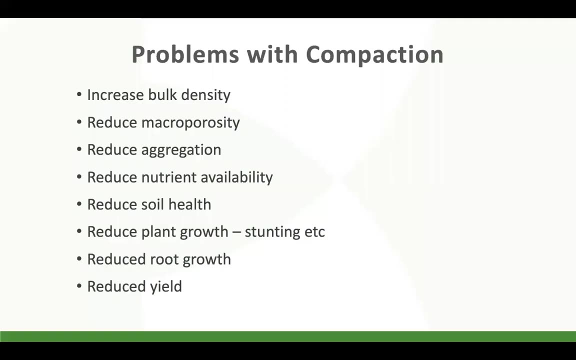 Maintaining aggregate stability is key to preventing erosion And, ultimately, we are decreasing the stability of the particles when they come together. If we, if we, if we are able to achieve this, then we're able to do this. they're very dispersive if they break apart very easily. this is creating conditions that are 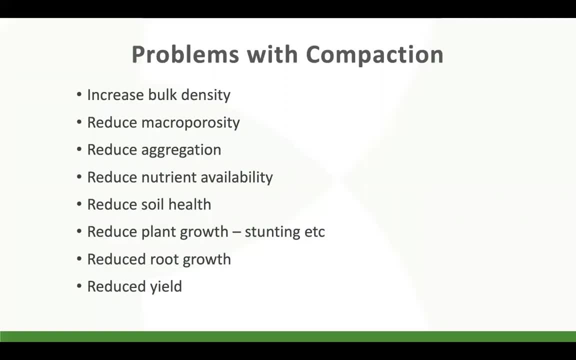 optimum for for soil erosion. so, um yeah, this is just summarizing some of those kind of points that we just went through on that more detailed slide. but we increase bulk density. that really reduces the porosity, particularly the macro porosity, reducing aggregation. that's going to. 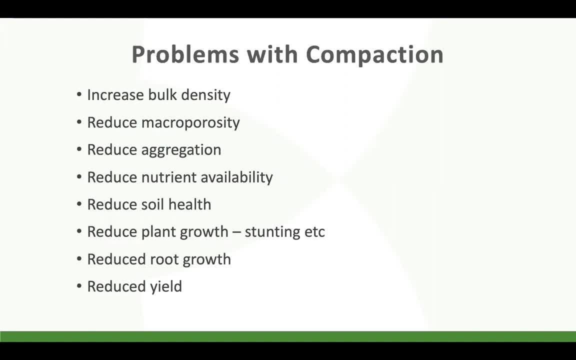 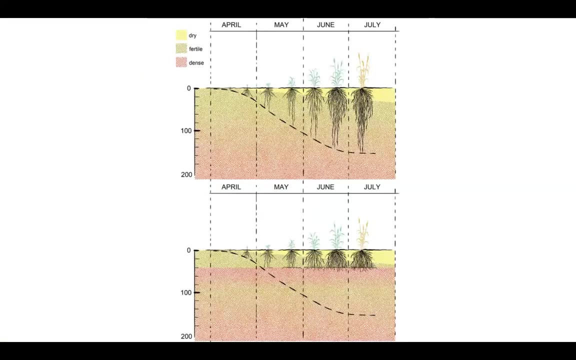 reduce nutrient availability to the plants. this is all. these things are contributing to reductions in soil health, ultimately reductions in plant growth, stunting root growth and overall, ultimately reducing yield. and so you know, this is kind of the. the image on the top is what we would normally see in an average year where, um, as the season progresses, as the plants, 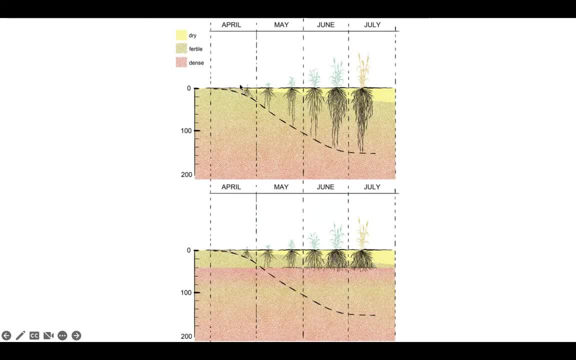 grow that. of course we have a small seedling that gets started and as that soil- sorry, as that plant grow in the soil- completely erесь. we then have rotrill and then allongar, myon, Dennis, Right. so in the middle of this week, on October 11, we did sort of a big shift on placing soil. Tell me your score. 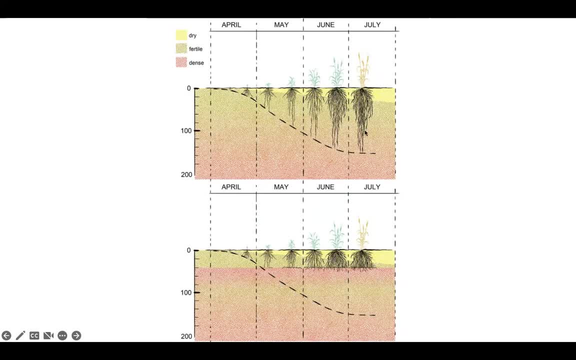 through the rest of the season, through to maturity. you know we have, by the end of that stage, we have, you know, decent root production, particularly at depth, when, when the plant is able to penetrate through there. however, if we have a tight and compact layer, that is going to limit. 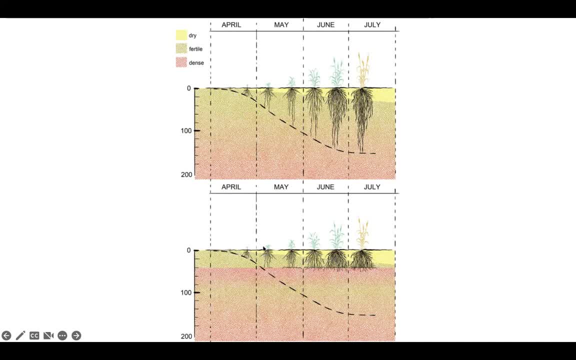 this red layer here that is going to limit root penetration as that season progresses. of course, as you can see, the roots just are not getting down to their full potential. and if they're not getting down to their full potential, of course they're not accessing moisture, obviously. but 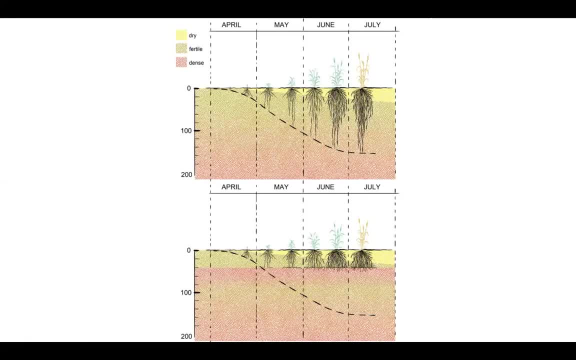 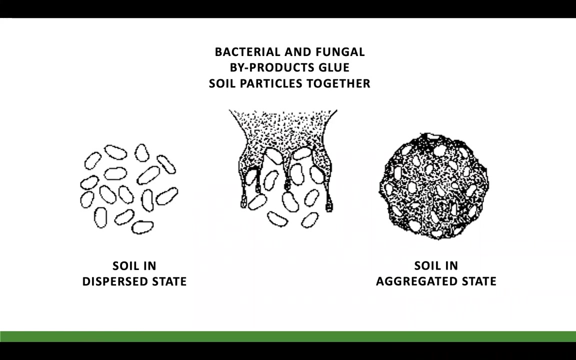 they're not accessing nutrients as well, and so those are two key ingredients that plants need from the soil in order to to grow, and so, of course, once we limit root growth, we limit moisture and nutrient supply, we're going to limit production potential above ground, and so this is what i mean when i talk about aggregates- improving soil aggregation. it's 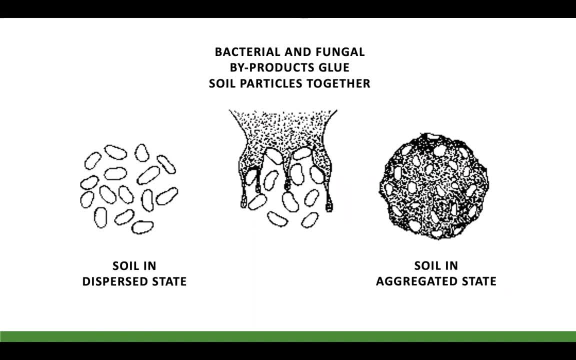 really about the the positive side of pulling the soil particles together to create these nice aggregates. and when we create those aggregates, what we are creating by default in between is these pore spaces, the space in which water can penetrate, that oxygen can come in, the co2 can come out. it's all about that porosity in the middle between these and these aggregates and 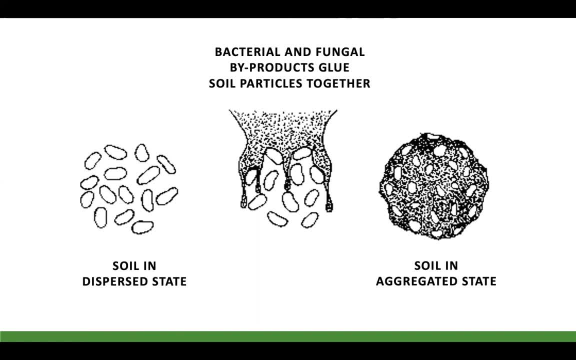 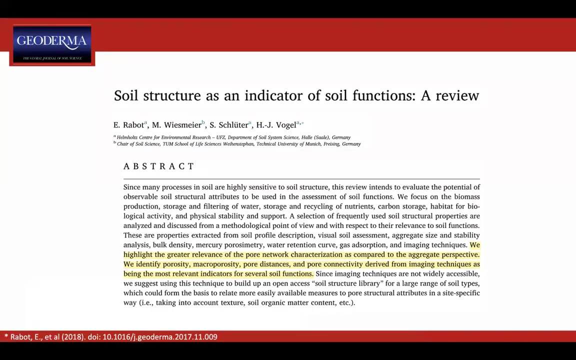 and really the key driver of aggregation is roots and the associated microorganisms that live with those roots, particularly fungi, but but many of the bacteria and fungi. they are releasing these gluey type substances that help to stick and glue the sole particles together, aggregate those soils and therefore create the pore space in between. and i just 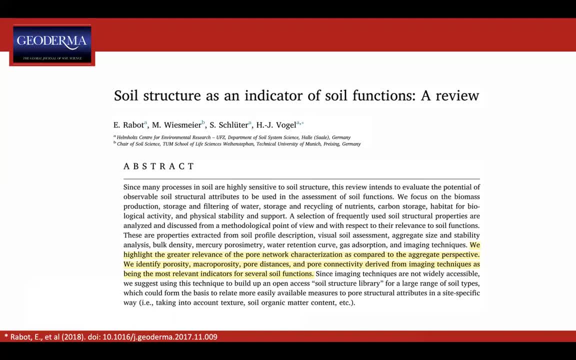 out of interest this study that was kind of looking at soil structure as an indication of overall soil, folding the shit we have for rail soil, cantonia, Hardwoodchuck soil, orbit, executor, kim function and, as they mentioned here, we highlight the greater relevance of the poor network. 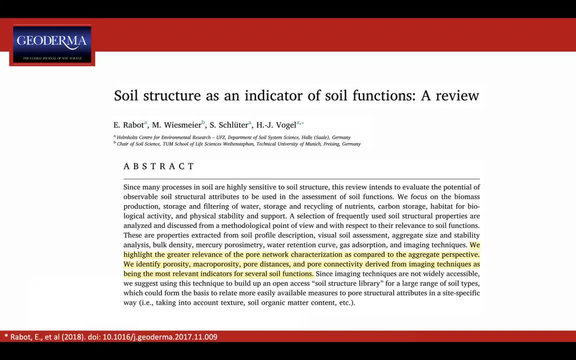 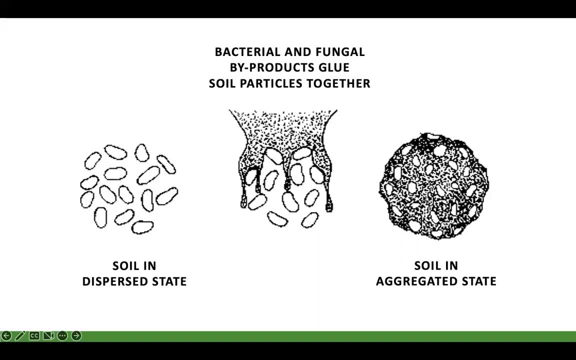 characterization as compared to the aggregate perspective. really, what they're saying is a lot of talk in the world of soil, health really focuses on on the aggregates and we want to increase aggregates, increase aggregate stability. they're really important for capturing carbon, sequestering carbon and, of course, all of this is true. aggregates are really important, but by default, when you 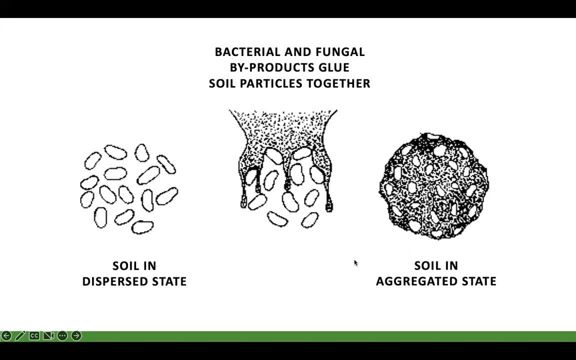 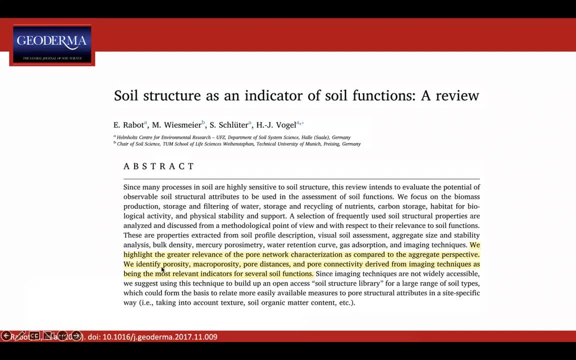 aggregate soil, you are also creating the pore space. they're, they're yin, they are yin and yang. you know one and the same thing. um and so, as this study is pointing out that actually they identify the porosity, the macro porosity, the poor distances and particularly the poor connectivity, how well. 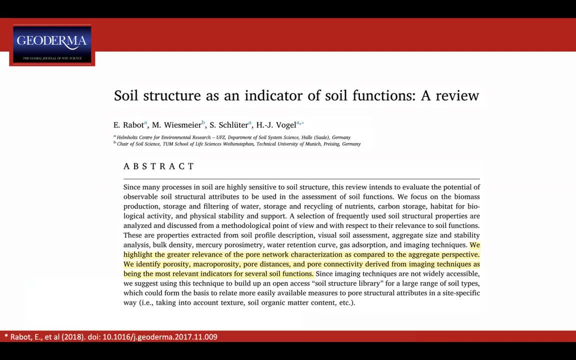 all of the pore spaces in the soil are connected um and derived from special imaging techniques that they. they identify all of these things as poor relationships, um. and then there are related traits as being much more relevant for several soil functions, so that there's much better correlations with how well the soil is, the, the porosity, the, those various 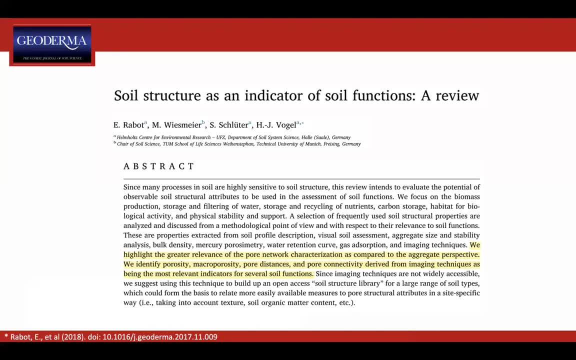 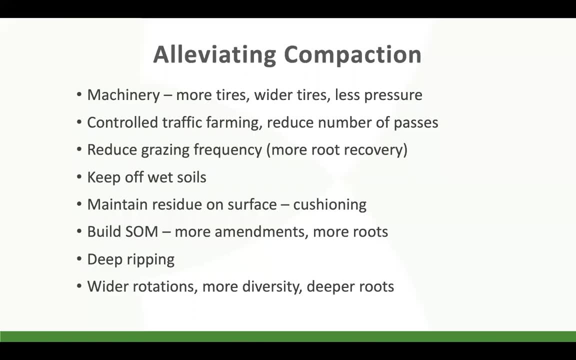 porous properties, that these are much better correlated to overall soil function than necessarily the aggregates. but but of course they are one and the same thing. so okay, moving on. how do we then alleviate compaction and address this issue? and okay, some obvious things. with machinery, the more tires, the better the 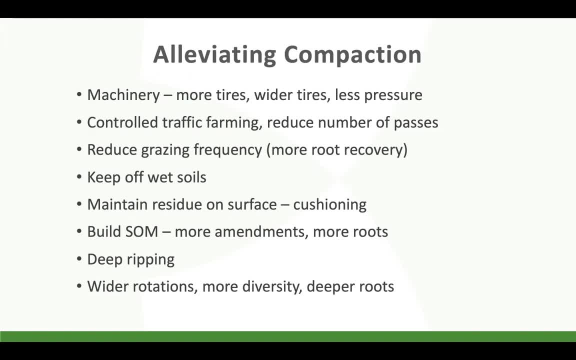 wider tires, the better, the less pressure. if you've got more and wider and less, there's less. less pressure, you've got less downforce. that's basically causing that compaction. so you're just evening out the weight distribution of the machinery, ultimately leading to less compaction. 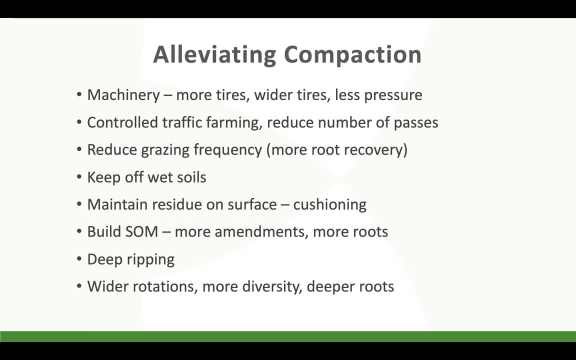 so more tires, wider tires, less pressure in those tires is good. equally, control traffic farming. so just trying to maybe maintain the same train, tram lines again and again. reduce the number of passes, if possible, also a good strategy. and then of course, with grazing we want to reduce the grazing. 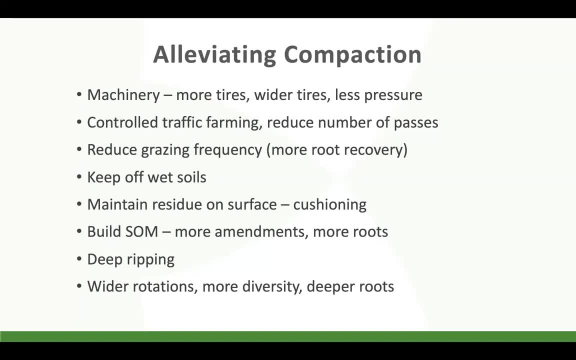 frequency. so if you can give the after the grazing event, if you can give the grass, the pastures, more time for recovery- when animals come back too soon is when we have the problems. so if you can stop divide your fields into smaller parcels of land and just keep those animals moving. 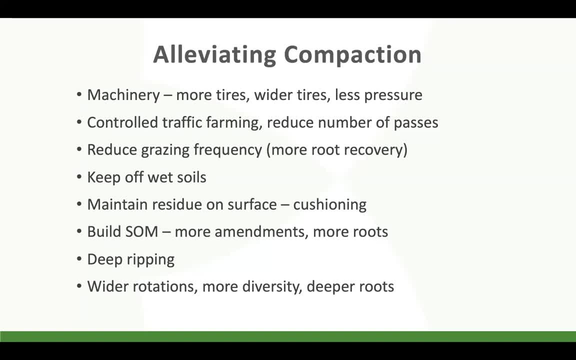 more frequently into these smaller areas, then just try and keep them for as long as possible before they return back to back to the same parcel of land, and in doing so, you are creating opportunity for more root recovery, which is is really what's going to prevent the compaction from. 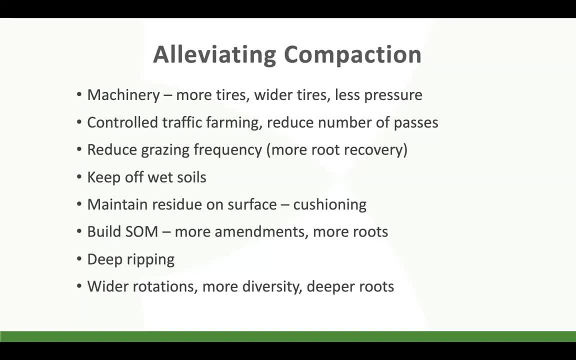 um, in the first place. and coming back, as i mentioned, keep off wet soils. absolutely. just don't go there. you're going to be causing more headache than gain, that's for sure. maintaining residue on the surface is also really important. this creates like a cushioning kind of sponge effect, so that 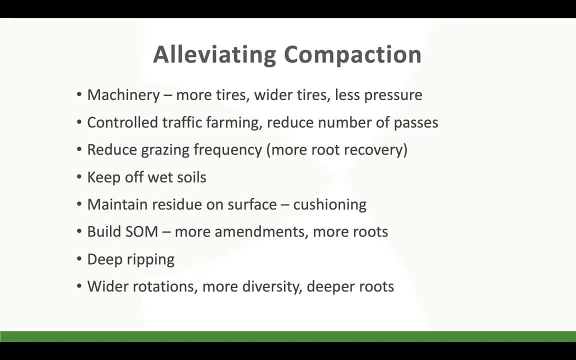 actually with good surface litter um. be that crop litters, stubble residue or grazing or pasture, a faction litters um. it creates a lot of damage to the soil. so it's really important to keep that um up humorous and it's really interesting to think about how we can possibly make the soil a more. 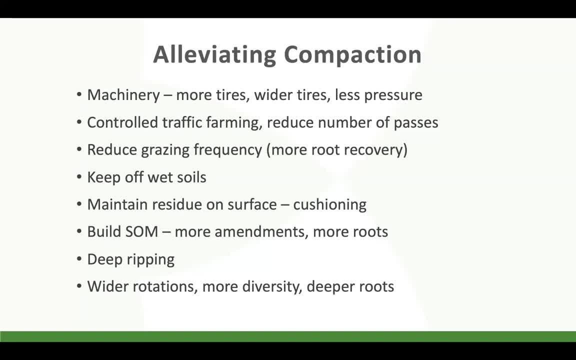 spangy, cushioning, and actually the soil can tolerate more machinery or more great or animal impact when we have a nice, um spongy protected, mulch kind of layer on the surface. um, you want to build soil, organic matter. i'll talk about this next. the more organic amendments: composts. 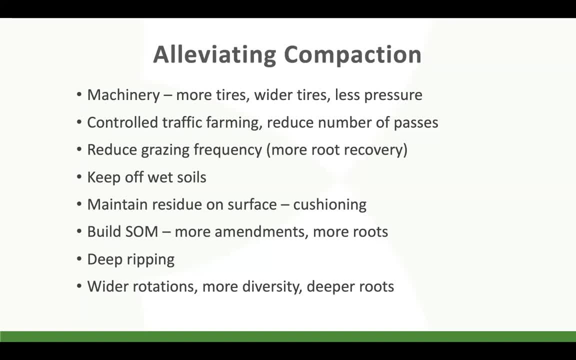 manures. the more roots you can grow, the more you're going to yield, the more you're going to drive. So that's going to help basically make the soil more tolerant against compaction, resistant against compaction. Deep ripping is also a strategy. It's you know, it's more of. 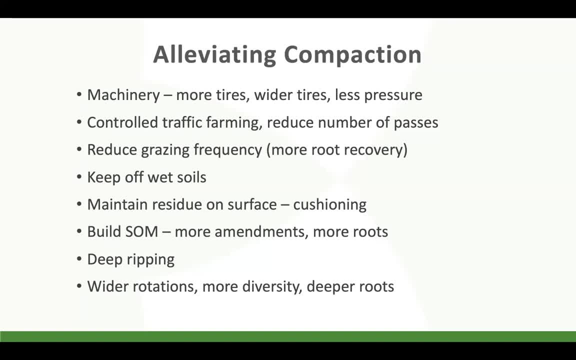 a treating the symptom than addressing the root cause. but that's okay as a short-term strategy. to just crack open some of that, the subsoil compaction anyway, and give the roots a chance to get down there, That's good. but that's the key point. The problem you have is not a lack of 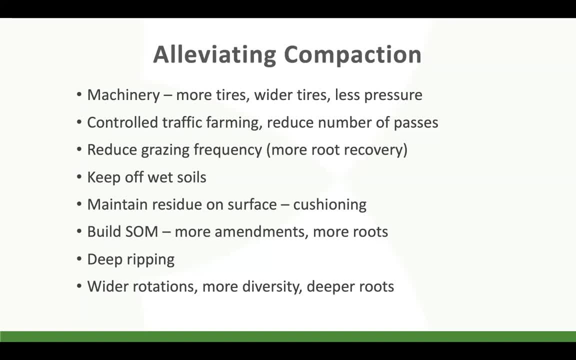 deep ripping, The problem you have is a lack of root. So if you're going to deep rip, fine, but make sure you get some roots down there to then slow down and prevent that soil from just really compacting again. So the real root cause of your problem is lack of roots. So let's work. 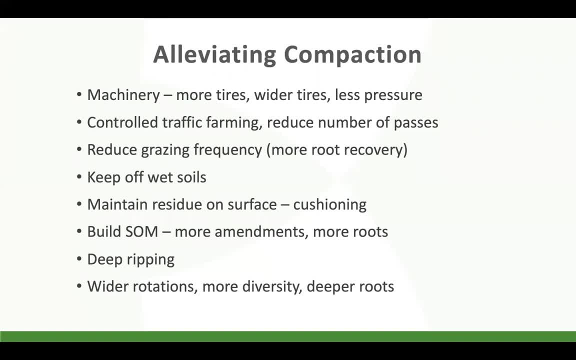 on getting deeper roots down To prevent the soil just from re-compacting And really then, in terms of again kind of prevention strategies and prevention being, you know, preferable than dealing with cure- just get more diversity, wider rotations, more diversity in the pastures, mixed species pastures. 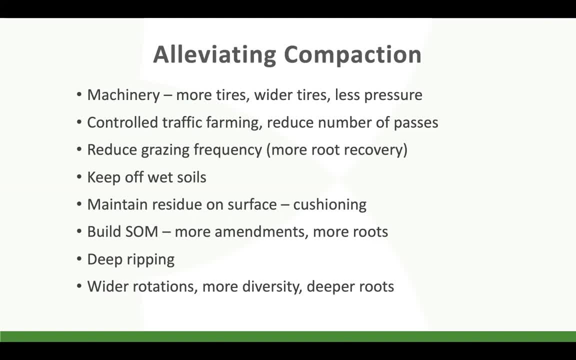 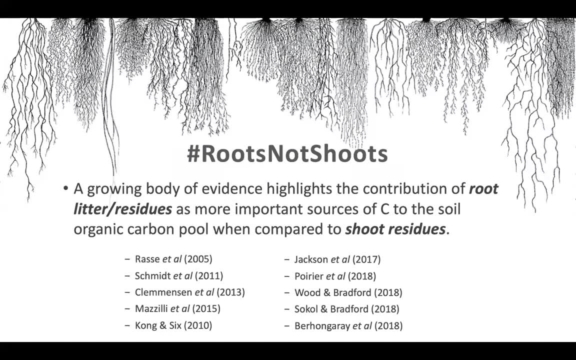 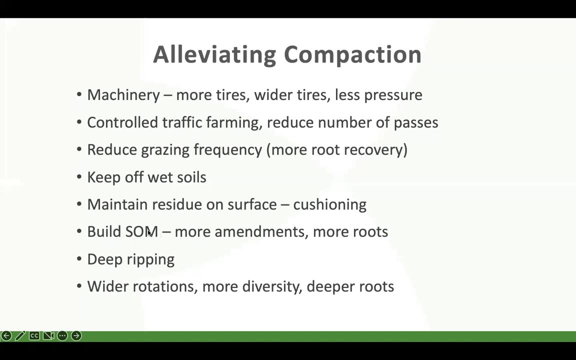 and choosing species that have nice deep roots. This is kind of going to help to prevent the problem in the first place. So let's have a quick few points about, okay, how do we build soil, organic matter, and just kind of cover some of the key areas on this, Because I think this is really a central point in this. 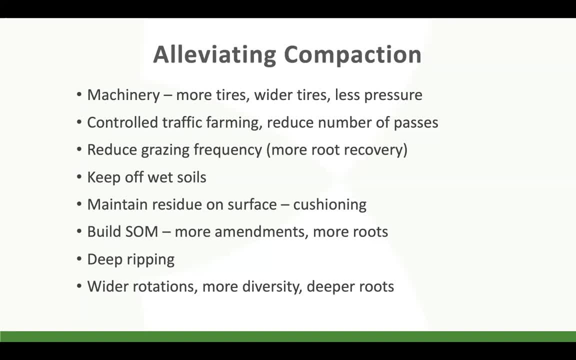 discussion. really, The more soil organic matter you have, the less prone you will be to compaction in the first place and the easier it will for you to be cycling carbon and building organic matter. So I think this is an area that is a very good preventative measure, So it's one that we should 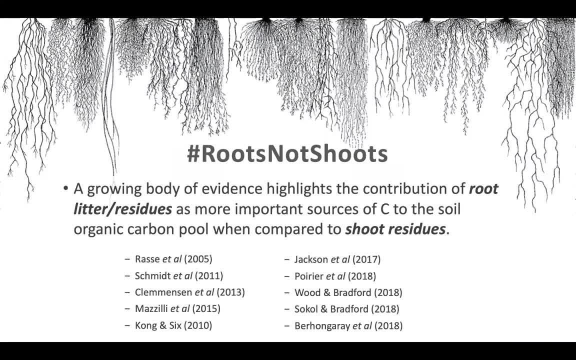 spend a little bit of time to quickly just focus on And building soil. organic matter in a way is an easy topic, but also a very complex topic. Ultimately, we just want more carbon in the soil, And sure you could do that if you've got the 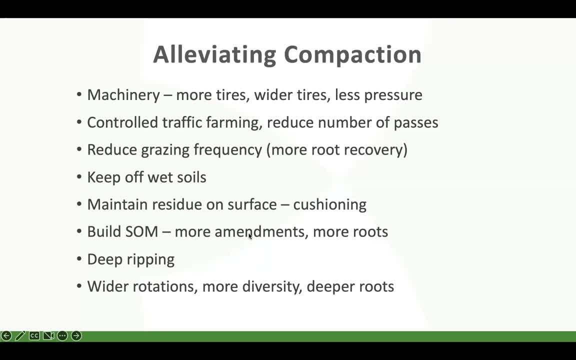 resources with simply adding more manure, more compost, just applying carbon to the soil. Sure, that's one way to do that and accelerate that, But really we want to do it primarily and more caustic, economically, through just growing more plants, more roots, more photosynthesis. 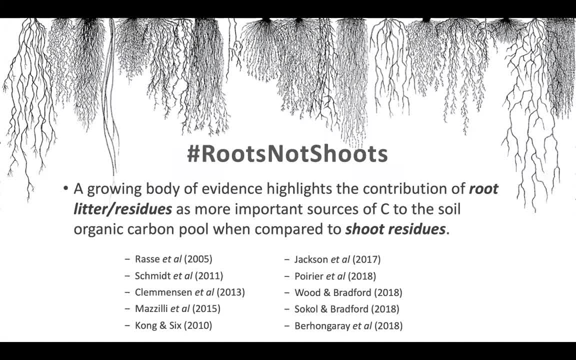 And the key thing to understand is that, in terms of building soil organic matter, it is roots and not shoots, So it's really the below ground biomass, not the above ground biomass, that is the key, primary driver of building soil organic matter. We have lots of studies that have 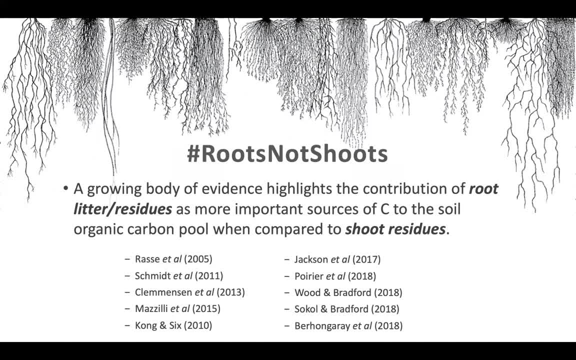 really compared shoot litter as it decays in the soil and root litter as it decays in the soil. And roots are much more important. If you want to build soil organic matter, you need to grow more roots And, of course, if you want to address compaction, you also need to grow more roots. And 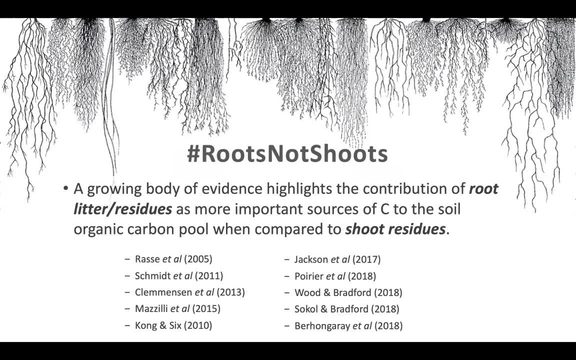 there's no surprise to that. These things are very interrelated or they're all intertwined very much one and the same thing. So there's many studies. all really support this, And I'm just picking out one here. Jackson, this is a review study, So it's a study that simply reviewed all 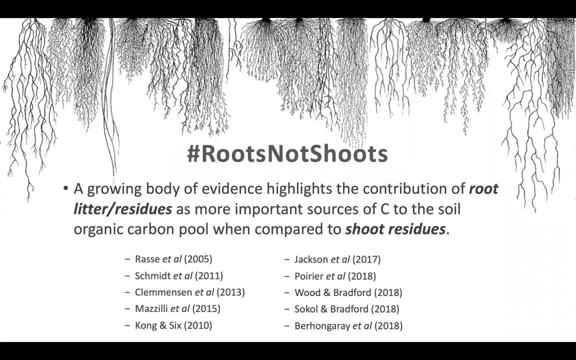 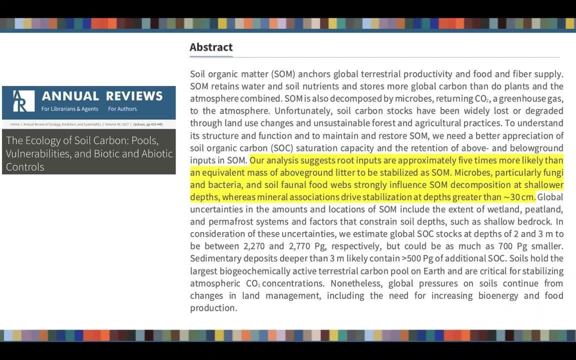 of the lots of other studies and kind of summarized the overall findings. And as they point out here, our analysis suggests that root inputs are approximately five times more likely than an equivalent mass of above ground litter to be stabilized as soil organic matter. So roots- 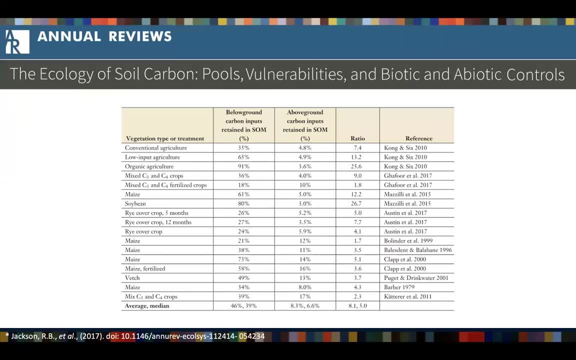 therefore, are five odd times more important than shoots in building soil, organic matter- And this is a summary table where this is many of the studies that they kind of summarize, And we're not going to go through each of these, but just for you to scan your eye down. 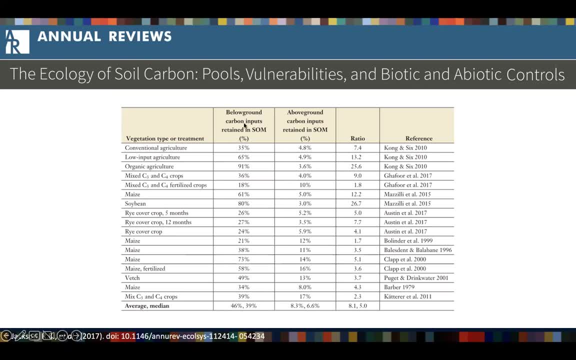 here we're looking at what percentage of the below ground inputs- so what percentage of the roots- were ultimately captured and turned into soil organic matter, versus what percentage of the shoots, the above ground residues, were captured and turned into soil organic matter. And, as you, 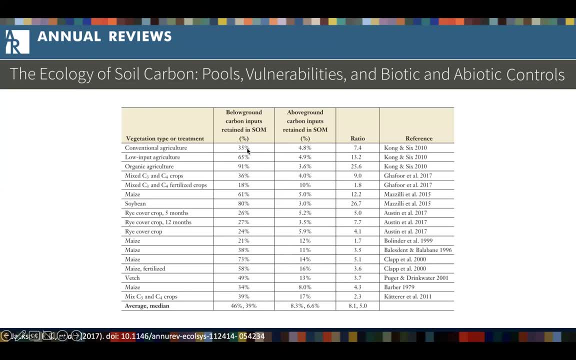 can see here that if you just quickly scan your eye down this list, what percentage of roots kind of became soil organic matter versus what percentage of shoots became soil organic matter, And you can see that generally the numbers here are much higher. And all of these kind of they've 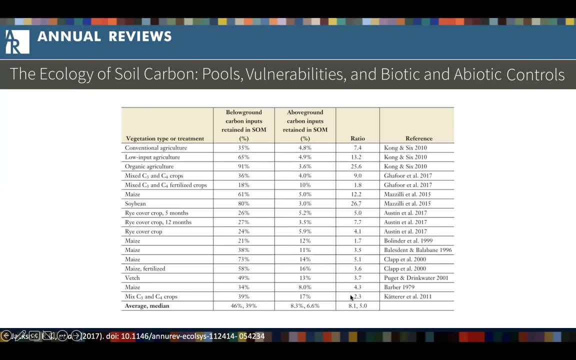 summarized this down to be that it's around this kind of five times more. you know, amongst all of the variability and the differences there- different soil types, different climatic conditions, et cetera- On average roughly rough rule of thumb soils, roots are five times more important. 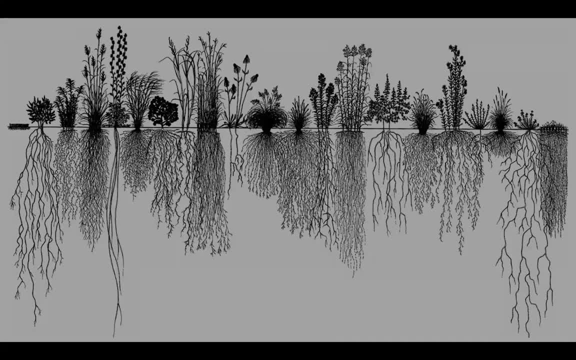 than than shoots in building soil, organic matter. So that looks like it's going to take a little bit more time And that's probably just to these this kind of point and say, okay, it's, what's really key is what's going on below ground. It's really the roots, not the shoots, And undoubtedly the best. 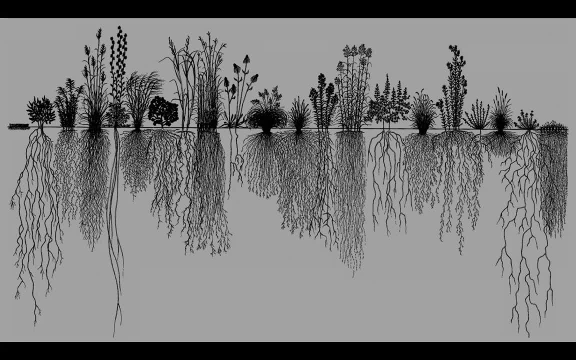 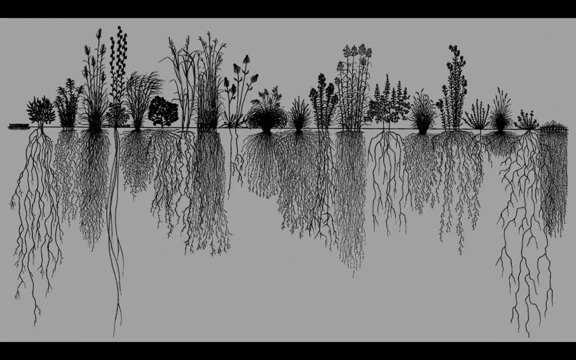 matter, but also prevent compaction. and, of course, when we then graze these plants- unlike in this depicted in this image, where they're all starting to go to flower and go to seed- when you come in and graze these plants and push them back to vegetative growth. 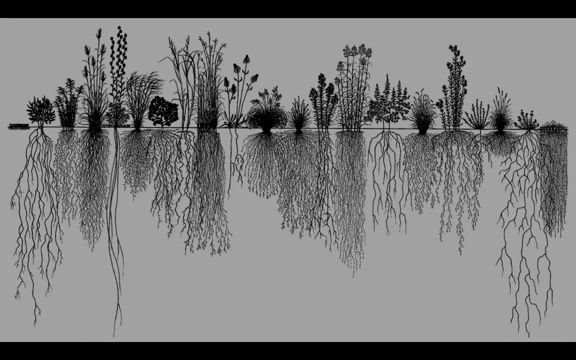 actually that's what encourages more root growth and more root exudates as the plants go to flower and go to seed, as you kind of see here. actually, this is where the plants then prioritize reproduction and they will send more energy and photosynthates and things up into the seed and 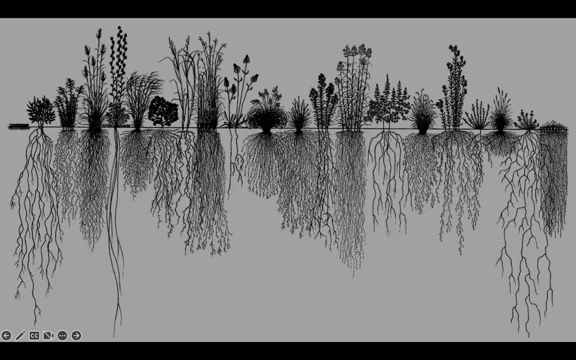 the developing grain and seed, etc, fruit, etc. so if you prevent them from going to reproduction, you keep them in vegetative stage and prevent the reproductive stage, then actually you're keeping the roots more active, keeping the roots turned on, keeping root exudation, keeping this process much more functional. so this is why 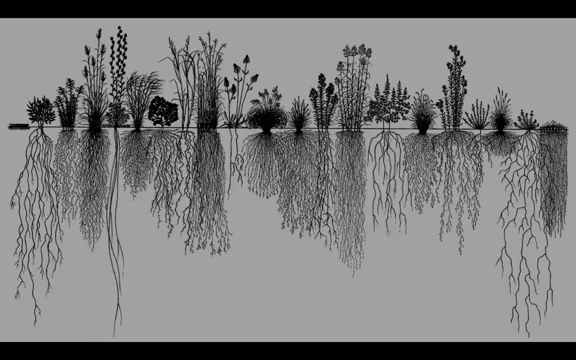 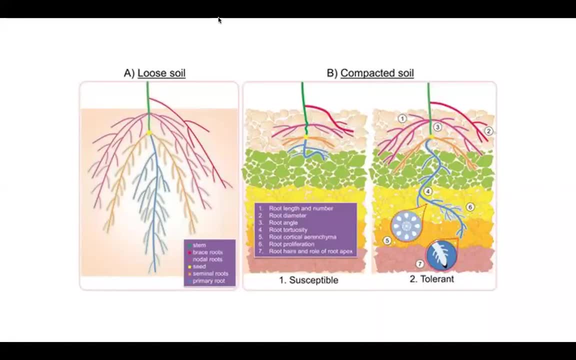 grazing animals on perennial plants is actually one of the best strategies to prevent compaction but also to build soil organic matter, and we have many plants that can be formed part of your tools in this kind of toolkit, and just to illustrate that you know, some plants vary. 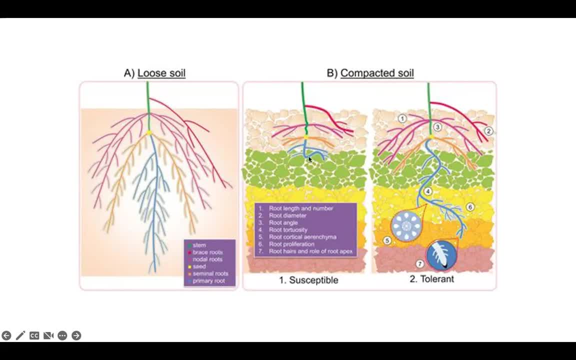 they're very susceptible to compaction. they just really don't do well. they just simply cannot penetrate, whereas we do have some that can, then maybe are called tolerant. sure, they may be not super happy or thriving, but they can tolerate it. they'll perhaps develop some kind of a tap. 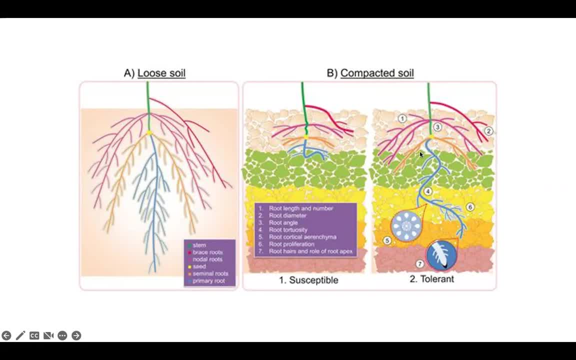 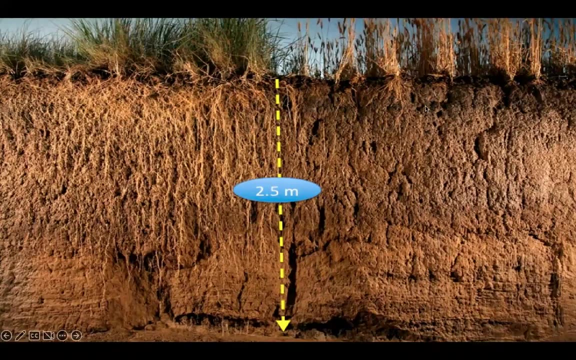 route that can get through those compact layers and still maintain some level of plant health or plant productivity kind of thing, as compared to these highly susceptible plants. and so, yeah, it's perennials as compared to annuals, perennials, they allocate more carbon below ground. annuals do not, and so wherever you can get more perennials and particularly deep rooting species, so you know things like alfalfa is a good one. timothy poxfoot, you know, plantain chicory, some of those tap rooters, this kind of thing, just any of those. kinds of plants that can get more carbon below ground annuals do not, and so wherever you can get more perennials- and especially if they're perennial, but even if not, just some of those deep rooted plants are great, and they do a much better job as compared to our annuals, who 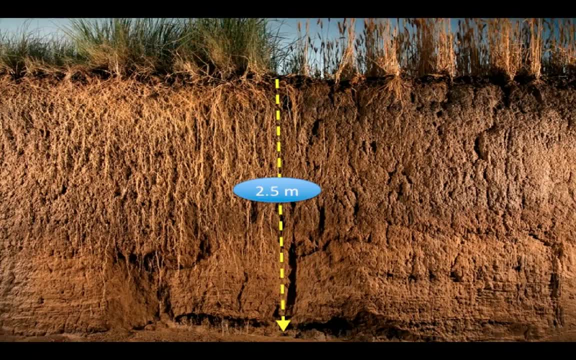 don't get me wrong, annuals can play a role too. annuals are very quick to grow, quick to establish, so they can be kind of very good primers of the soil, prime the system quickly and they can be quickly and early in spring and early in the season and the perennials can kind of finish the 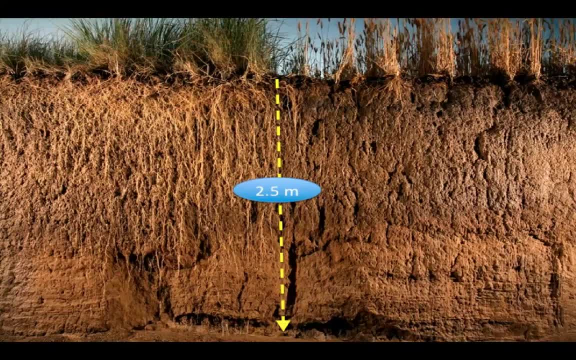 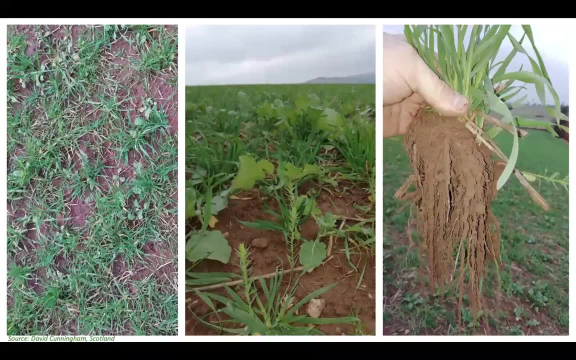 job later in the season. so there's a. it's not that annuals necessarily are all bad, but they definitely work better in in tandem in concert with, say, with some perennials. and just an example: here you're looking at a cover crop. this is quite. this is from scotland, again quite a northern. 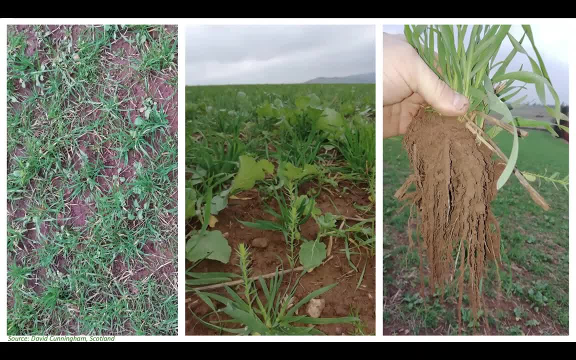 climate. it was late in the season, november, and you know this was a cover crop. you might look at this cover crop and say, well, it looks pretty good, but it's not. it's not good, it's not good. it's pretty small. there's not really much biomass above ground, a few inches tall. maybe this doesn't. 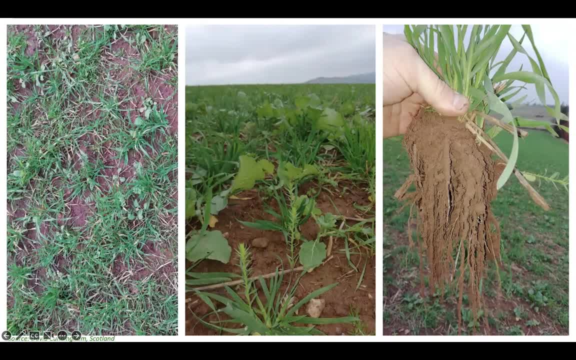 look so impressive, but actually it's not just about what's going on above ground. it's also about what's going on below ground, and that's where the roots are so key. and so, if you really want to assess cover crop health, take the spade and have a look at the root system, because this 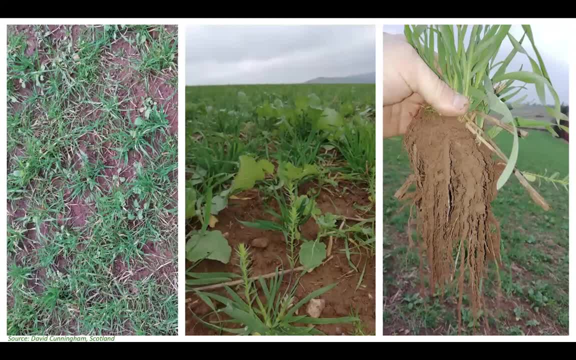 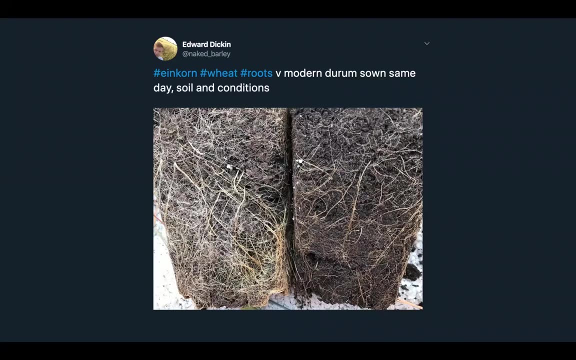 is the same soil, same photos, same day, and you can see that actually, although the plants are not so big and showy up top, they're still producing pretty good roots down below. and one small other example just to highlight that even amongst annual plants, some have better roots than others. even some varieties have better roots than 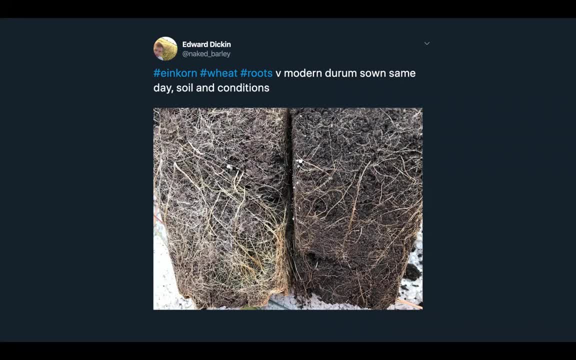 others. and here you're looking at einkorn wheat: on the left, the traditional heritage kind of cereals, versus a modern durum on the right. and this is just the potting soil: same soil, seed sown the same day, same growing conditions, Etc. and you can see clearly that einkorn wheat has. 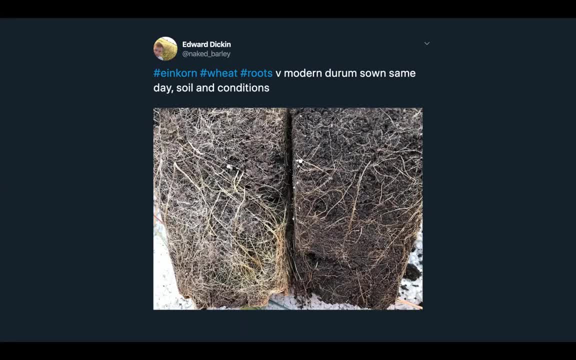 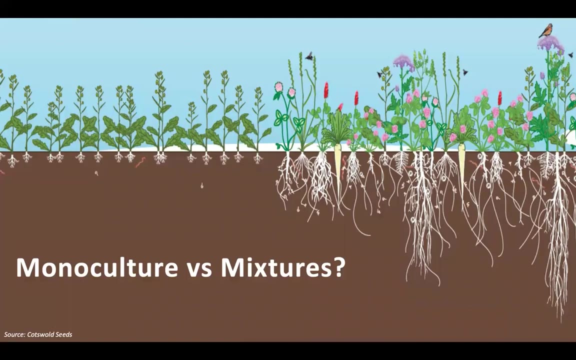 hugely allocated, much more carbon below ground, growing much more roots and therefore much greater potential to address compaction and to build soil organic matter which prevents compaction. so there's a lot of opportunities simply there to grow more roots, and really then the opportunity comes with diversity too. 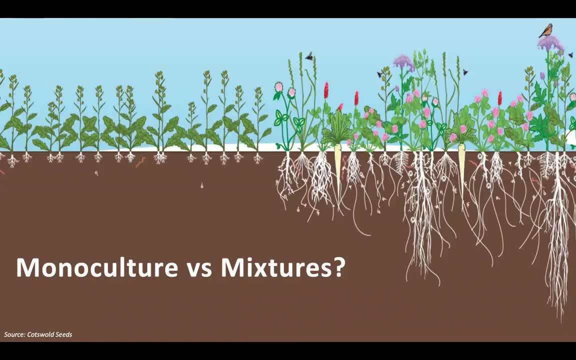 um with diverse roots. you have different species again, different rooting depths, different specializations of some of these different species. it's very complementary growing habits. you know, this plant is feeding in the shallows, this plant is feeding in the depths. so they have, they're not competitive, they are very complementary. they're not competing for resources, they're feeding in. 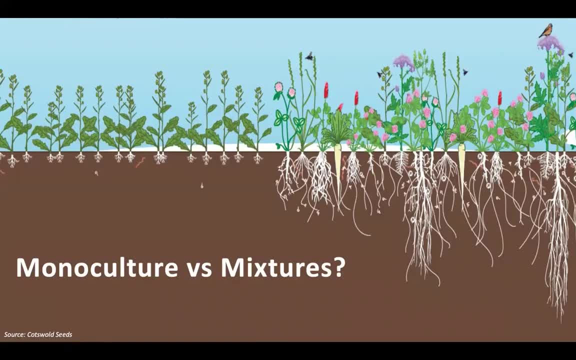 different areas. they're therefore complementing each other and therefore not maximize and optimize biomass production and growth accordingly, without limitations to to yield, Etc. so diverse roots- as again a picture says a thousand words. you can see on the right hand side just deeper roots. you can choose specific plants that are tolerant of, um, uh, you know certain soil. 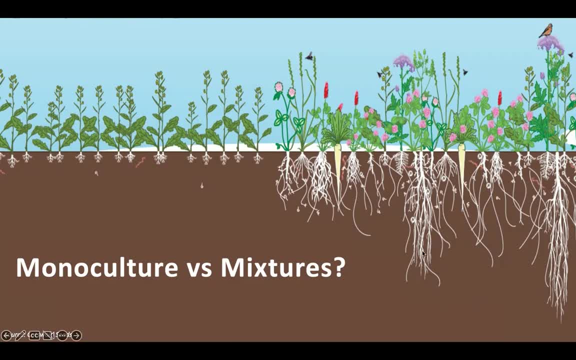 conditions. dry conditions, therefore, which means they're growing deeper roots so they can keep their production on under dry conditions. um, some others might be more shallow, but they have advantage of being quick out of the ground, quick, early establishment in the spring, when conditions are still cool. so you know, having 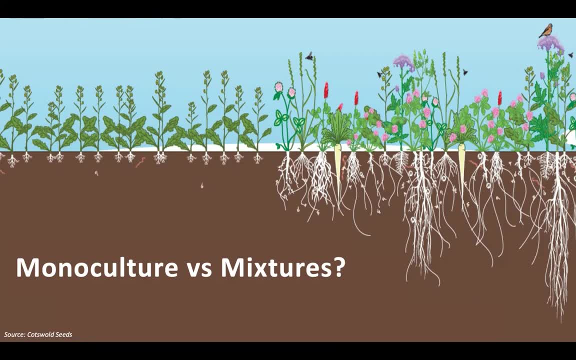 a mixture there creates this opportunity to hedge your bets and to at least always have something kind of growing somewhere in the field, amongst the field variability, or amongst the variability of the season, be it cold, warm, wet, dry, et cetera, et cetera. so there's real strengths. 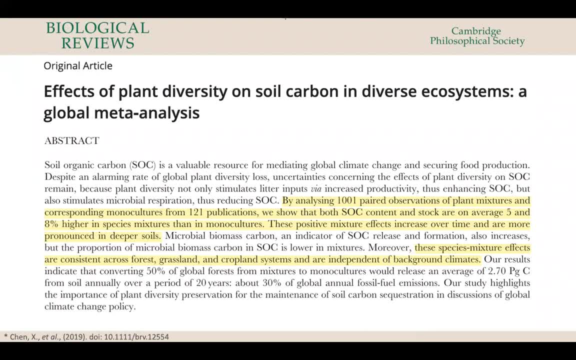 in numbers in in that sense, and just very quickly, um, talking about how important soil carbon is, well, plant diversity also helps to build that soil organic matter, and here we have a study that is- uh, was was exploring this question- the effects of plant diversity on soil carbon, and this is 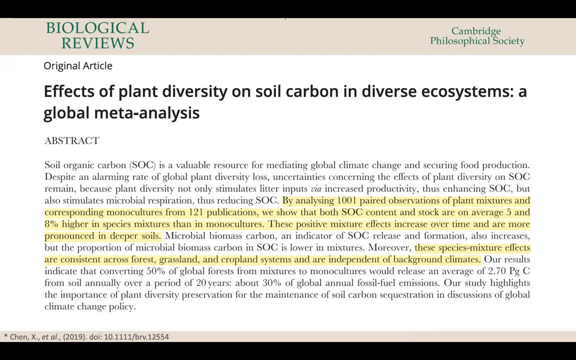 a meta-analysis. so it's again a study that just analyzes all the other studies and re-analyzes them, summarizes them, finds the overall kind of trends and patterns and that kind of thing and um. so here, as they say, by analyzing a thousand and one paired observations, comparing plant. 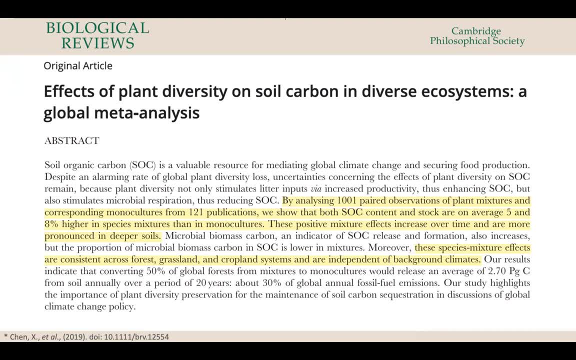 mixtures to monocultures. from 121 publications, we show that both soil carbon stocks and soil carbon content are, on average, five and eight percent higher in species mixtures than in monocultures, and that these effects were consistent across forests, grasslands and cropping systems. and 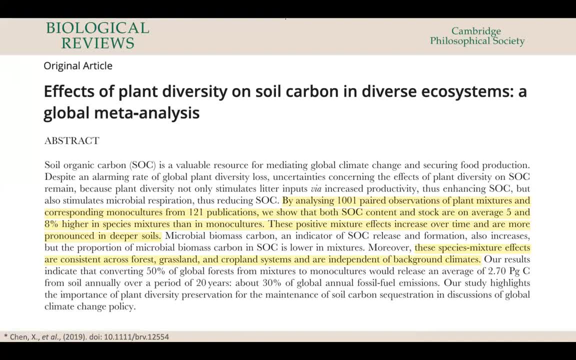 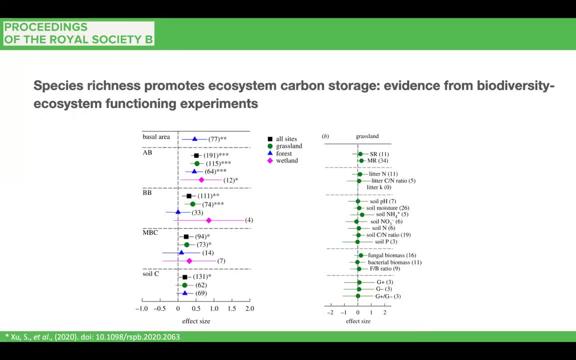 irrespective of all of them, the various background, climates and soil types and variability and all of that kind of thing. so so diversity seems to help soil carbon. here's another study that was saying, again a review that was staying the same thing: species richness promotes carbon storage. and so here we're looking. 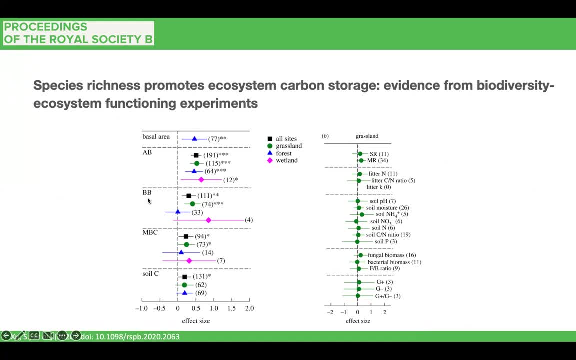 at above ground biomass, below ground biomass of the plants, microbial biomass, carbon and ultimately soil. carbon and everything to the right of the dotted line means that it's having a quantitative effect. so you can see that, indeed, plant species diversity increases. above ground biomass in grasslands, forests and wetlands. below ground biomass improvements microbial biomass. 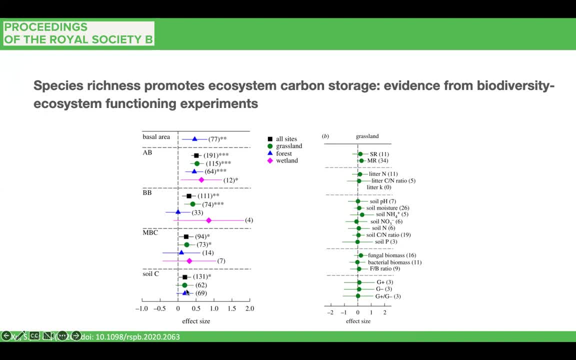 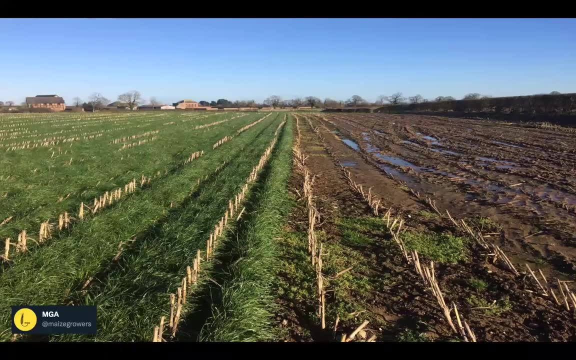 improvements and overall soil carbon improvements with plant diversity. so integrating more plant species diversity is very advantageous and you know as as much as that is the case that I would support that again like a nice picture which says a thousand words here. but here we have, you know, an under sown maze, just under sown with some Ryegrass, and sure, this ryegrass is just cheap. 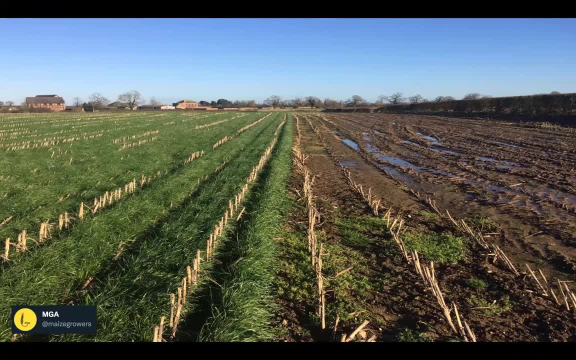 seed ryegrass. it's not a diverse mixture, it's just the monoculture of ryegrass. if I had a choice versus the left or the right here, I would absolutely still go with the left, you know, having just simply the soil covered and having a living root protecting. 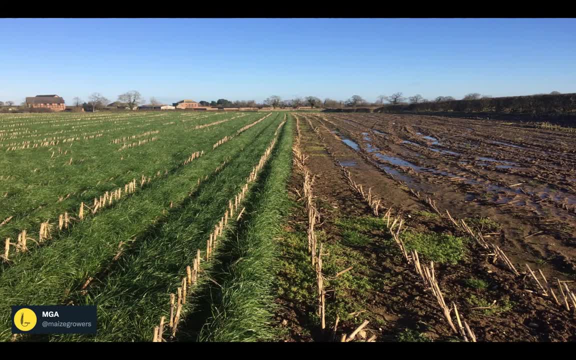 that soil and then having living roots and those roots growing, growing down to, to structure that soil, to feed the biology, to glue those aggregates together, to get that water down and into the soil. yeah, i would take it absolutely. so it's not to say that we have to have these extreme diverse. 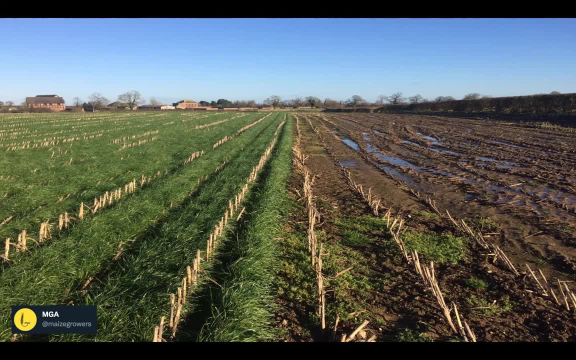 mixes either. i think some simple mixes is quite okay. okay, monoculture cover is certainly better than no cover at all. um, so again, it's all relative, but so this is great, but sure, maybe a little bit more diversity in here would be good to maybe at least maybe three or four or five. 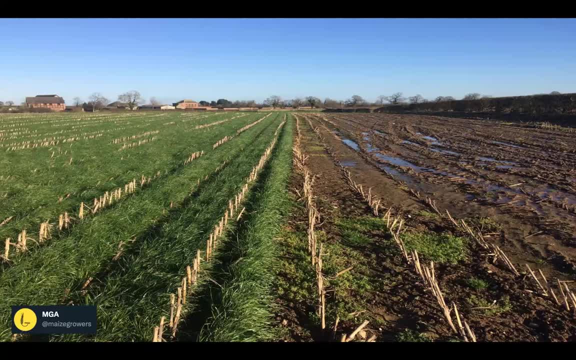 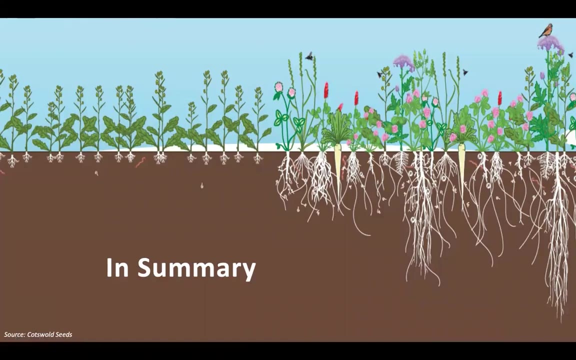 species, maybe just a couple extra, um, but again, just a nice visual image of just keeping the soil covered, protect the soil and keep those roots active. and you're not, you're going to avoid all of these kind of problems. so, in summary, this is my last slide back to this one, um, just to say that, really, soil compaction, of course it is a big issue and 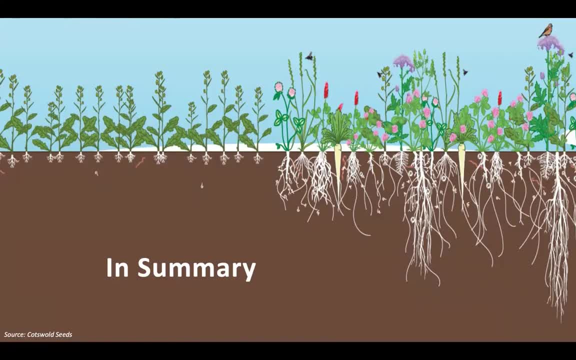 actually a huge number of agricultural soils are suffering compaction in many parts all around the world. it's a huge contributor to soil degradation and really the essence of the problem is really those roots that we've kind of talked about, emphasized quite a bit here today and and really 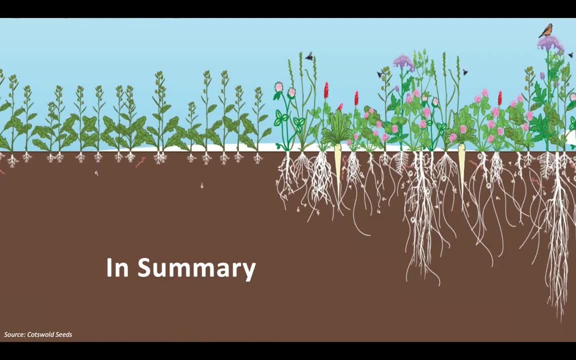 you know. you know it's not as much as things like deep ripping and machinery can be useful tools to address the symptom, they're not addressing the root cause. and the root cause is monocultures, a lack of agro biodiversity, a lack of deep rooting plants- um, you know choosing. 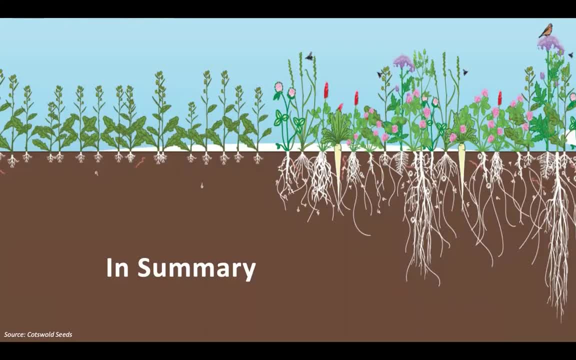 varieties that are very good yielding, and don't get me wrong, that's important too. we have to feed the world and all but um, when you choose varieties that are very high yielding, that that's a trade-off. it comes at a cost to root production, that's it simply means. 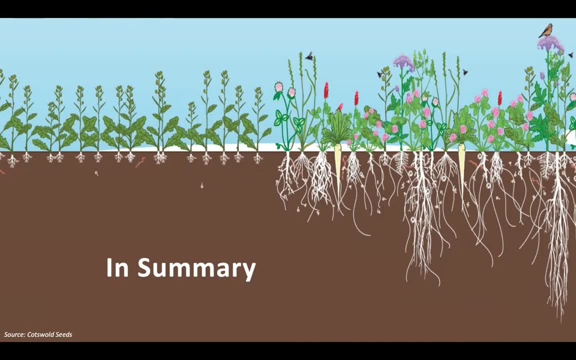 the plant is pushing more above ground biomass and not so much below, so it's not growing many roots, it's growing lots of shoots and lots of yield. and okay, i know you've got to pay the bills and get an economic gain, so of course that's important, but it's just about striking that. 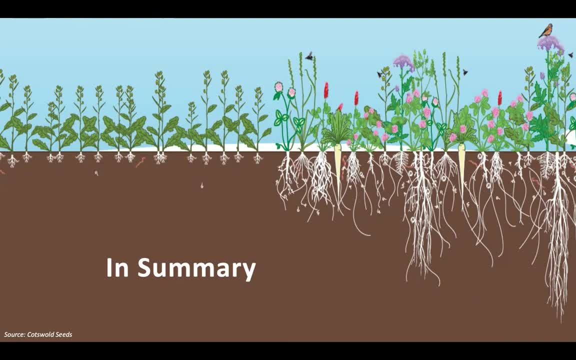 balance? um, we just need to grow more roots and more diverse roots. and sure you know, the problem is that you can break up some soil compaction, use machinery to address symptoms, but you've got to get roots growing back down there as well. roots is what's going to prevent. 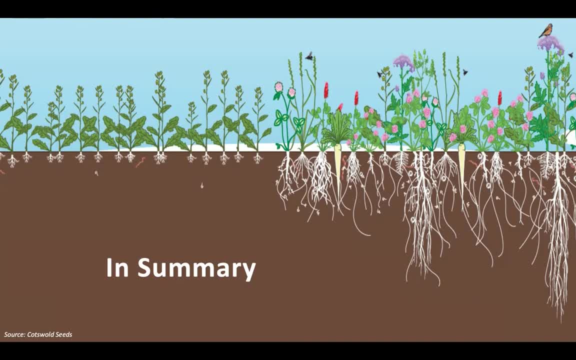 the problem from just coming back, and so therefore considering how we could transition to to more diverse roots, um using deeper rooted species, i think is key. so even in cropping situations, even going to two species is beneficial. intercropping, companion cropping, um- you can have a, you can have a. 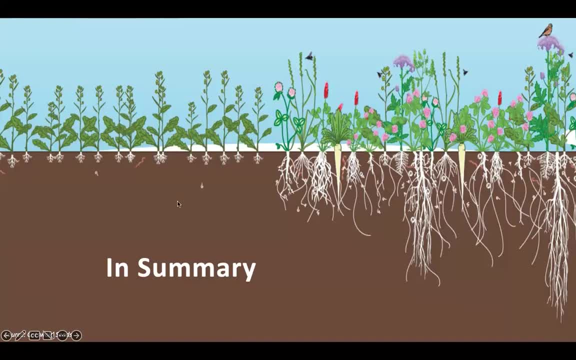 you can have a companion in in these inter-row areas, that whatever could be, this uh, tillage radish, the daikon radish, you know. put something in the middle that's growing down. uh, that's complementary, not competitive. just put something small uh on the surface, but deeper rooting um, and use the resources. 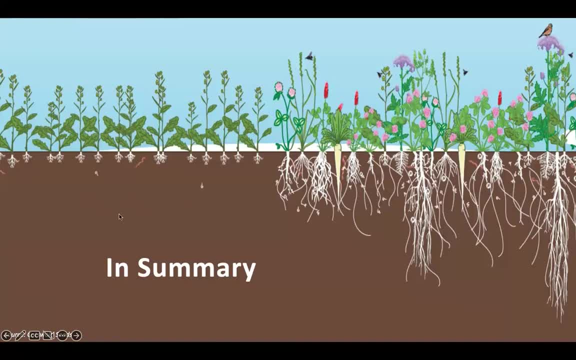 down here, capture water and nutrients, cycle them, uh, etc. so even in a cropping situation we can, we even just two plant species, but of course in a pasture or a cover crop situation, sure you can go beyond two. um, you can go to three, four, five or ten or whatever. um and uh, get these diverse. 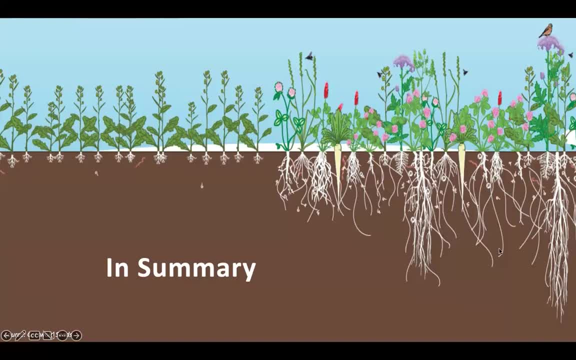 roots, uh, functional there to to prevent all of that soil slumping and compaction ultimately. so i think, in summary, it comes back to this point about roots and, um, that's really where the focus of your work is, and i think that's really where the focus of your work is and i think that's really 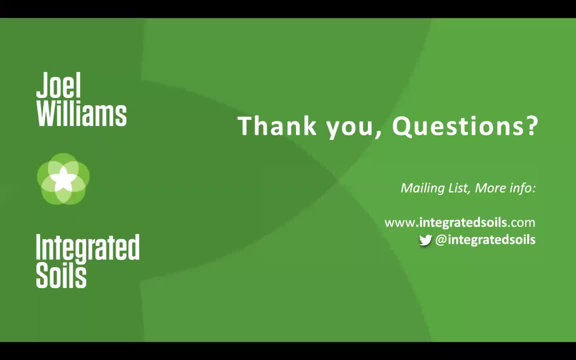 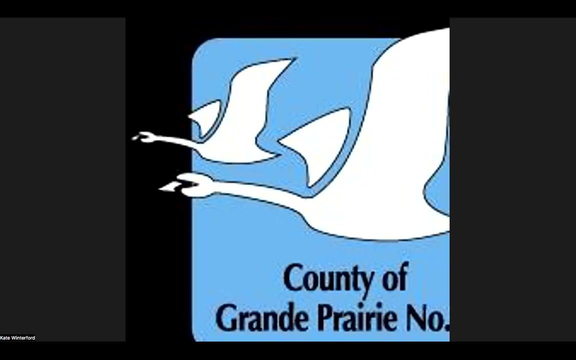 your management really needs to be okay. thank you very much. let's um have a couple of questions. if there's a few, yeah. if there's any questions, you can feel free to unmute yourself, or else, if you'd like to just enter it in the chat, you can do that as well, and i can read them out. 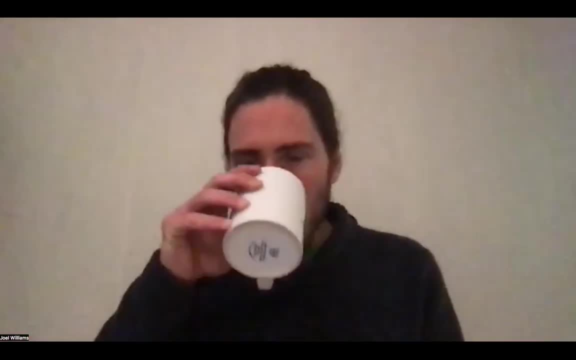 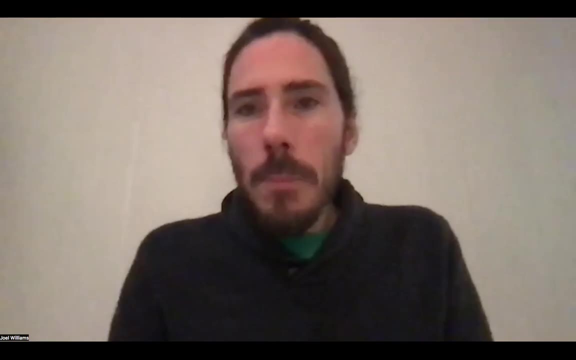 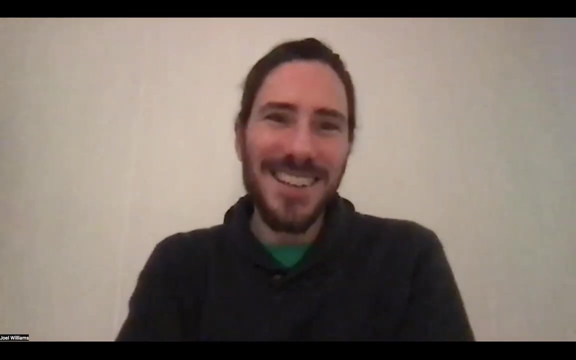 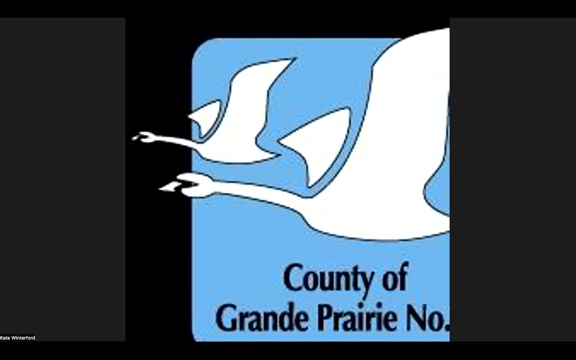 it doesn't seem like there's any questions tonight. no, everybody knew, everybody knew this already. well, if there are no questions, then i'll just remind everybody about um next week's webinar, tuesday, december 6th, uh, where we'll be doing a little bit of a little bit of a talk about the 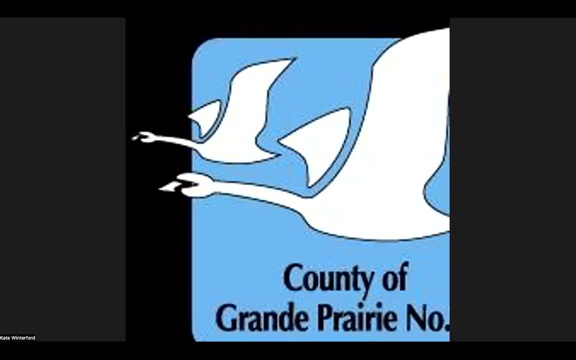 next week's webinar and then we'll be focusing on soil erosion again. this webinar will be uploaded to our county youtube channel. i'm just going to drop that link into the chat right now, and the link that i'm going to put in is, um the playlist that the youtube page has for all of the 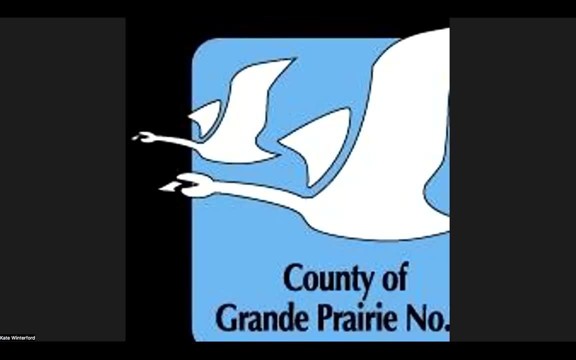 different agriculture webinars. so besides just the soil ones, you'll see some other previous workshops that we've done there as well. um, but otherwise, oh sorry, i'm going to go ahead and move on to the next question. um, sorry, we have a question. what about rolling soil for compaction? 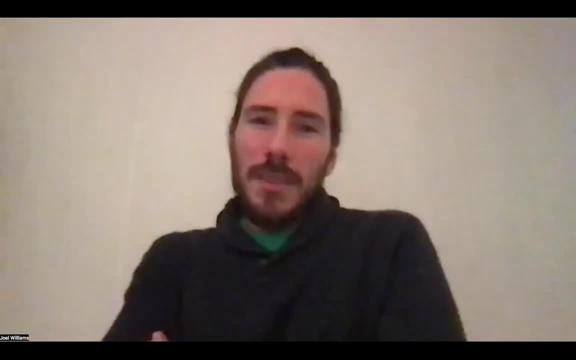 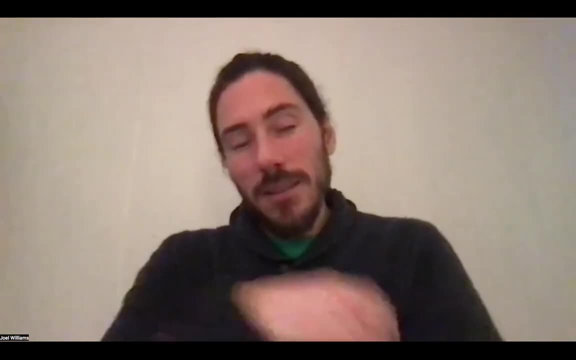 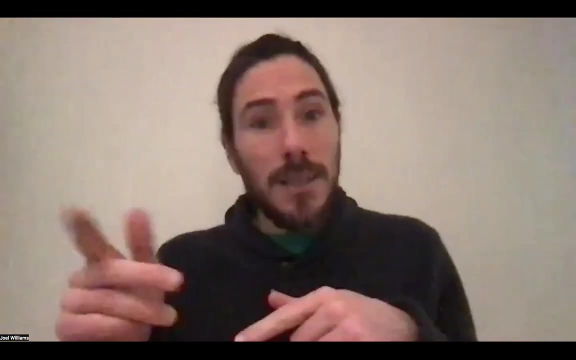 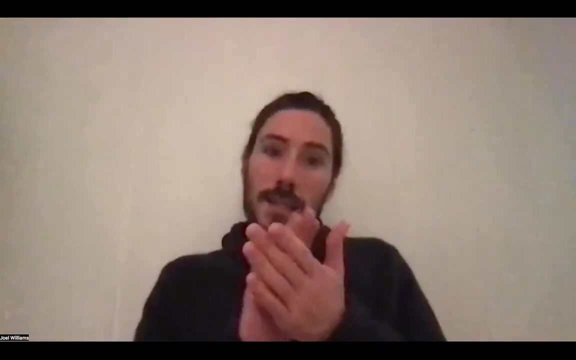 yeah, yeah, um yeah, interesting question actually. um, you know, often we would say that you know that rolling is somewhat important for compressing the soil a little bit, um, after seeding uh, to just make sure we get kind of a little bit of good soil contact uh with the seed. 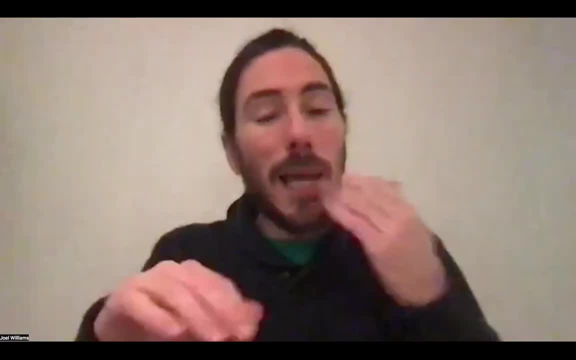 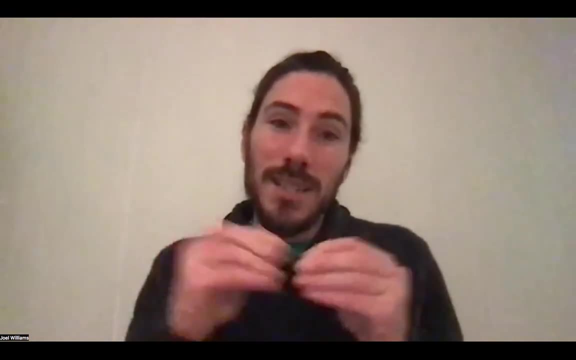 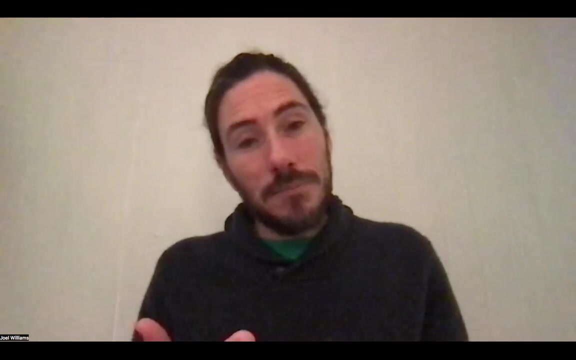 so it's, yeah, it's not uncommon to intentionally apply a light rolling, a light compression, um to enhance seed, seed to soil contact and therefore germination. so so, yeah, i agree, and you know, i was um, i was just in sweden a few weeks ago, uh. 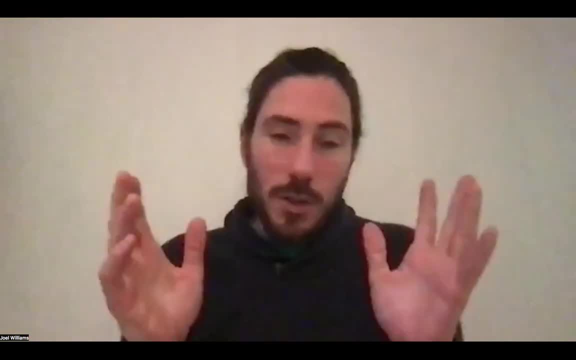 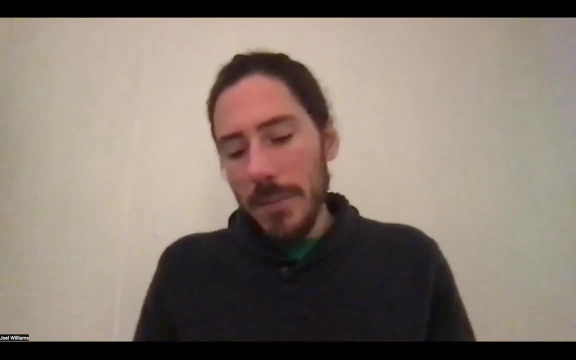 uh, giving a talk and i was also visiting a farm afterwards and, um, yeah, it was an organization that was doing a lot of work on the soil and i was just a organic farmer and i mean, i know it's in a temperate climate and you can get away with more. 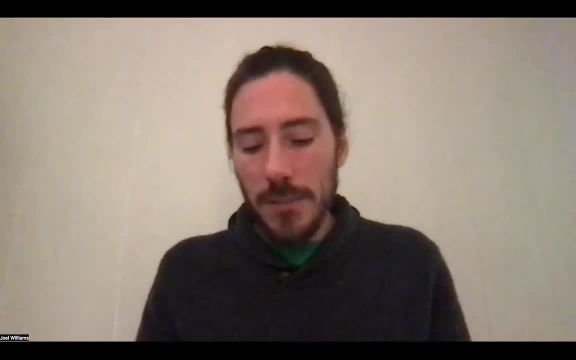 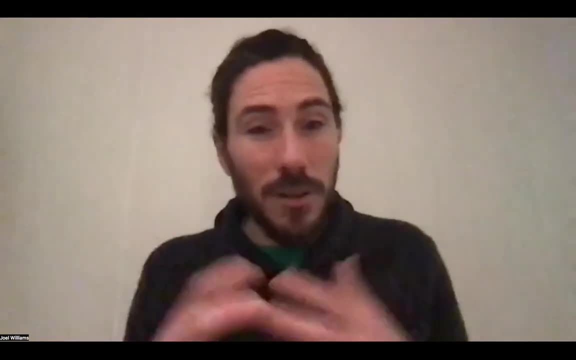 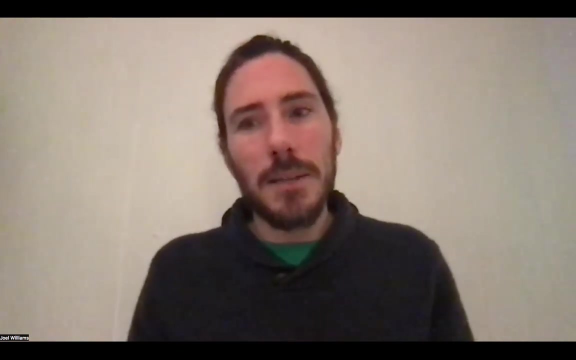 cultivations, uh, in those temperate climates versus the dry areas. but, um, i must be honest, he really challenged my views about soil cultivation, building aggregation and building structure with cultivations and, yeah, i was uh very impressed with some of the work um that he was doing and we are one of the things uh he was doing was applying some. 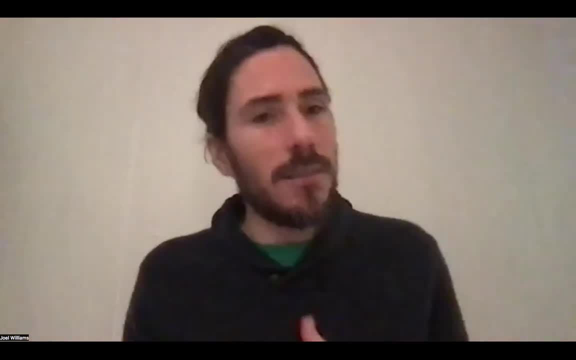 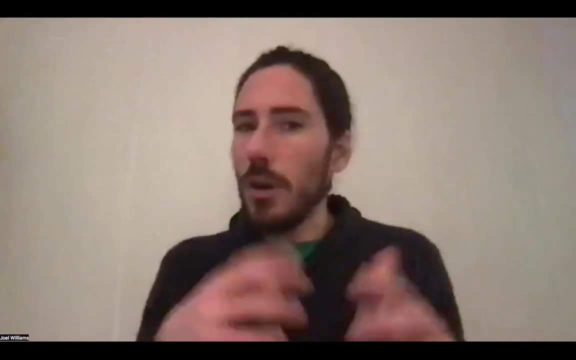 uh lactic acid bacteria, so some more fermentative bacteria which don't require oxygen, and a bit of an kind of an unusual technique to kind of integrate some cover crops with these fermentative bacteria. who will digest those? but part of the technique was incorporating them in and then 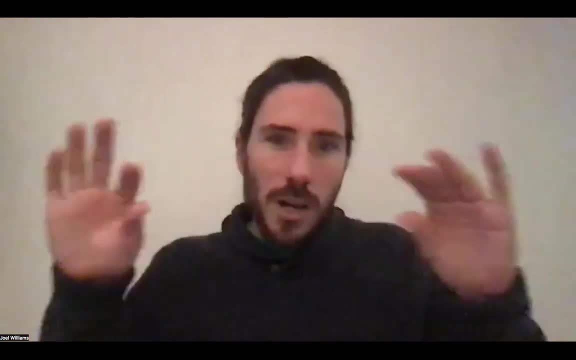 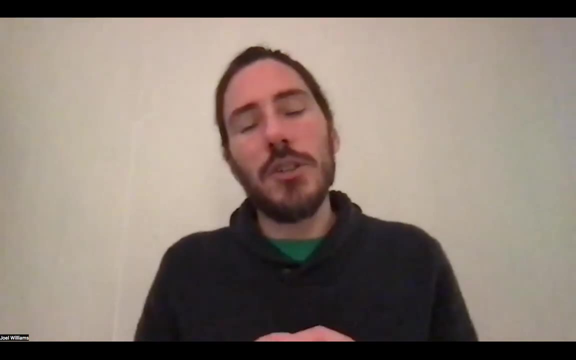 intentionally doing a compression, kind of almost trying, intentionally trying to seal off the soil to keep the oxygen out so that it could be more of an anaerobic style fermentation. and uh, then the soil would be more of an anaerobic style fermentation. and uh, then the soil would be. 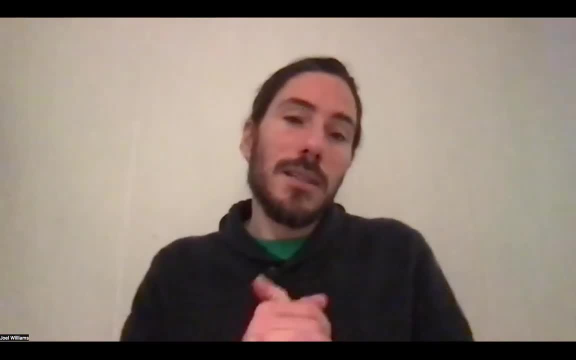 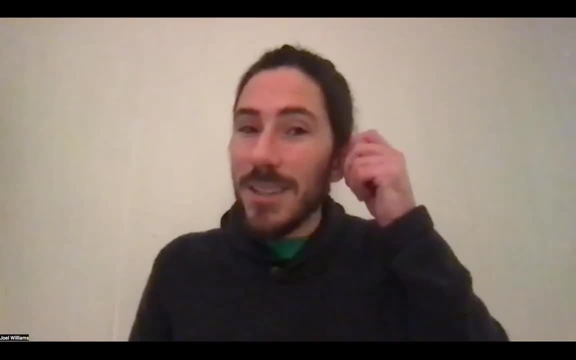 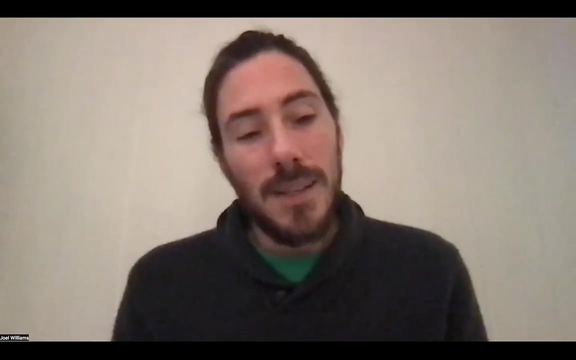 left to digest like that for around about 20 days, just under 20 days- and um, the soil goes through this incredible uh yeah, restructuring, digestion, microbially enhanced process and um, yeah, it really challenged my views- using kind of cultivation in these very specific and targeted ways that 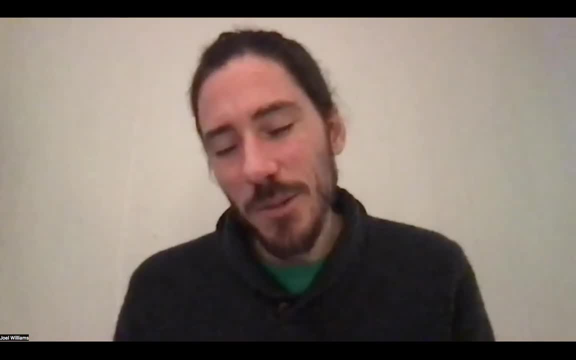 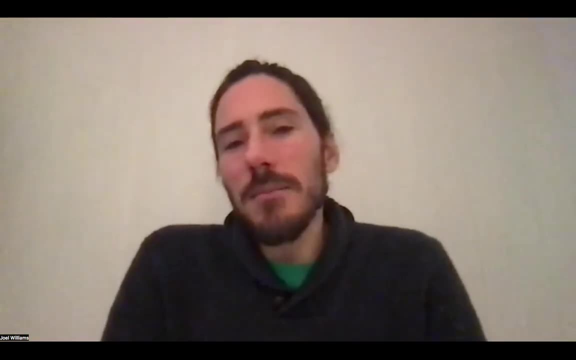 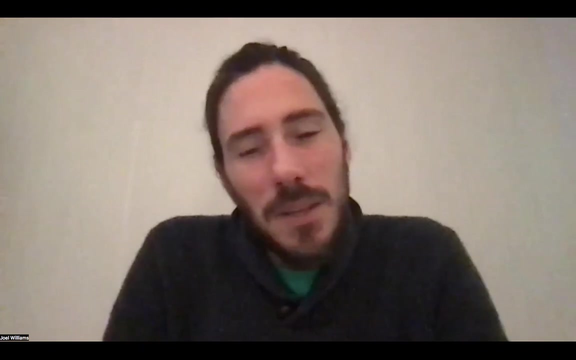 um, maybe can enhance soil structure and aggregation. so, yeah, i think there are interesting exceptions to the rule, like always, um, and i think that, um you know, some level of surface rolling or compaction is is okay, it's, it's all about you know how much it's. 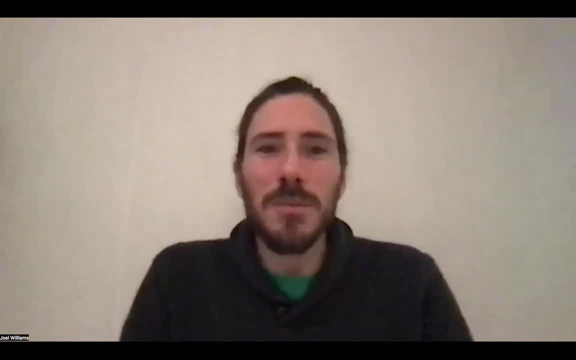 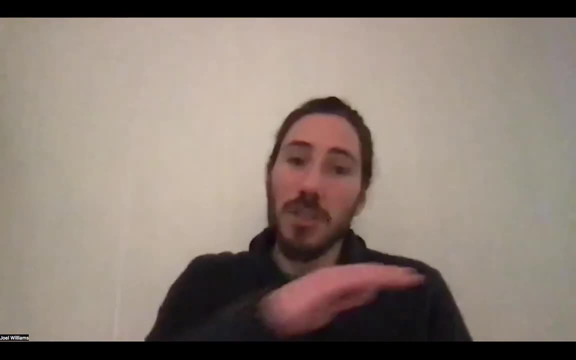 dose makes the poison. you know, if it's too much, you're going to cause problems, and we'll talk about that in next session. when we talk about erosion- because erosion is really- it's all about surface compaction, surface sealing and crusting, which is then what's really causing the erosion. 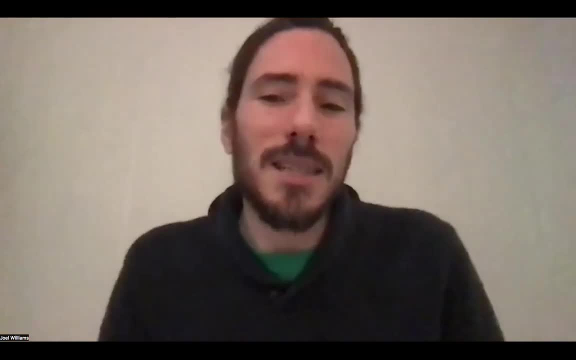 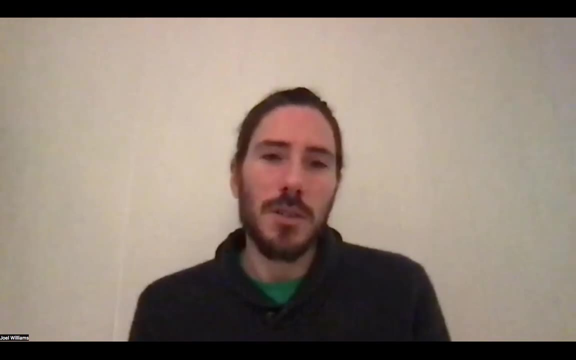 so we'll talk to that next week. um, but, but yeah, i think, uh, some small amount of rolling or surface compaction is okay. um, just not too much. okay, suggestions for improving breakdown of residue? yeah, yeah, okay. so that's. that's generally going to suggest a lack of biological activity. um, uh, if you're not getting good kind of residue. 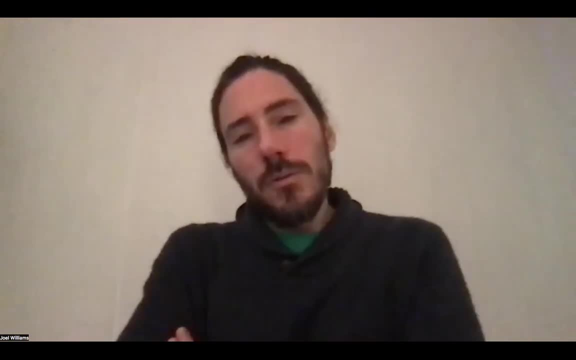 decay and and therefore cycle, so i think that's a good way to go about it. um, but yeah, i think there are some small amounts of rolling, or surface compaction is okay. i'm just not too much um cycling. so you've got a few options here you. it could be as simple as applying um some. 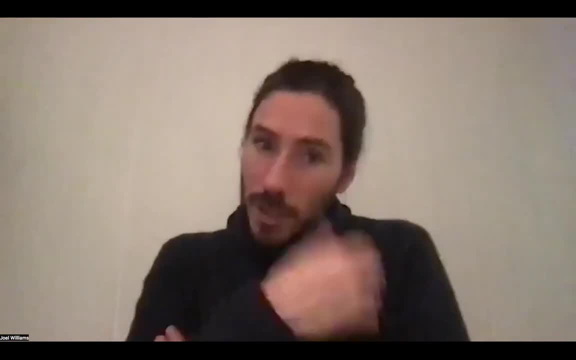 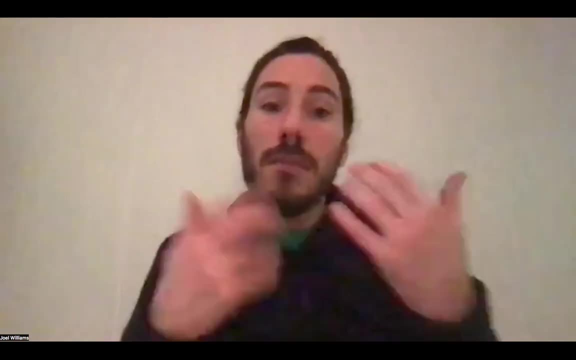 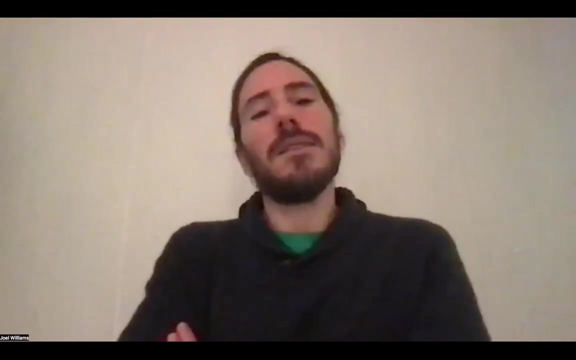 highly available carbon carbohydrates, food sources to just kind of prime the pump just to get the biology active to then digest those residues. and so what i mean by that is even things like molasses. molasses or seaweeds or fish hydrolysates these kinds of things, but molasses probably a more. 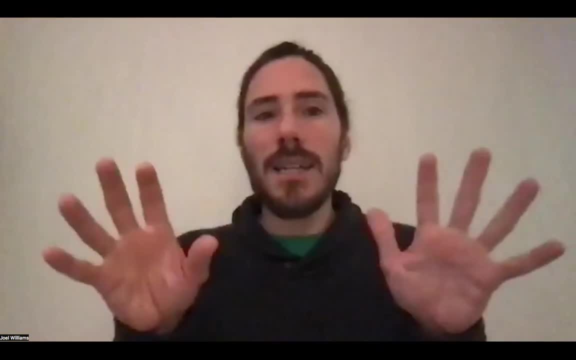 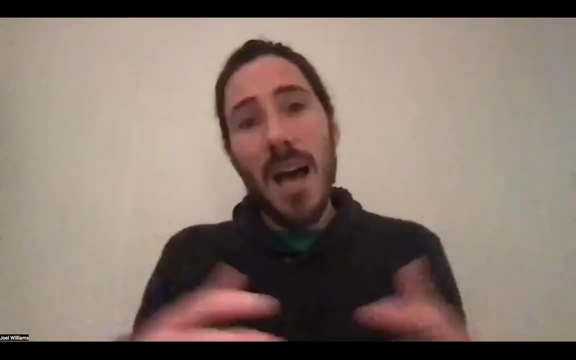 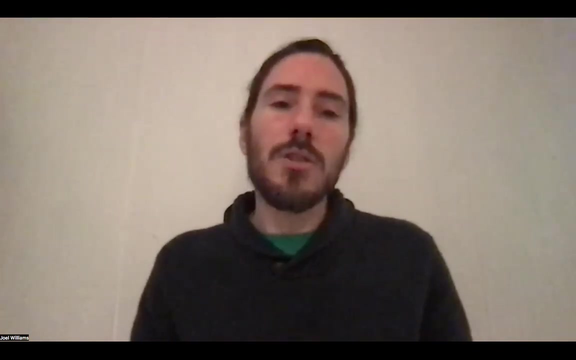 easier accessible one, and it just provides a highly available, highly labile carbon source for the microbes can kind of stop, excuse me that they can start feeding on and then carry on the digestion of um of the of the other residues. so so kind of priming the pump a little bit there. 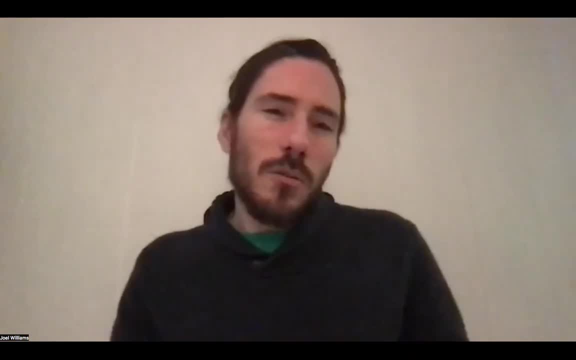 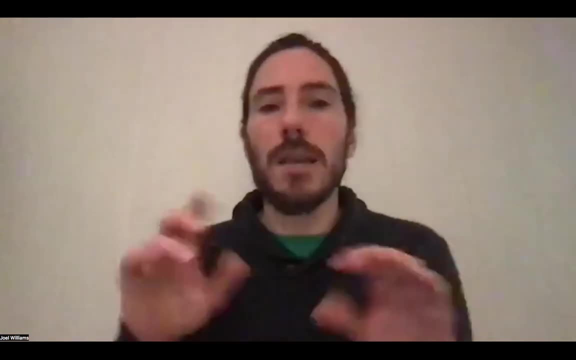 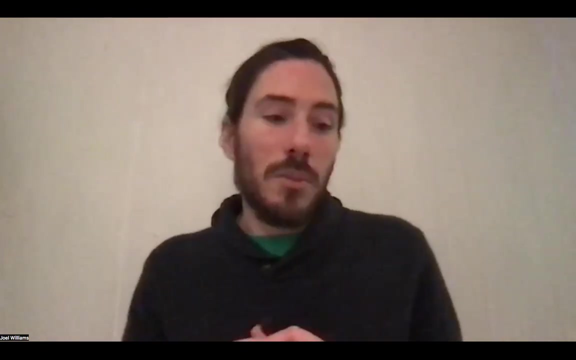 but also, um, generally, it's your fungi who are going to be a bit more important for some of that breaking down of some of the, the lignin and the cellulose, that more complex stuff. so trying to encourage them a bit also can help. so, um, using things like compost, fungal inoculants or compost extracts. 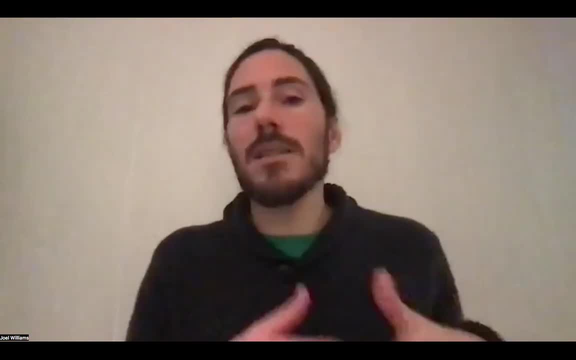 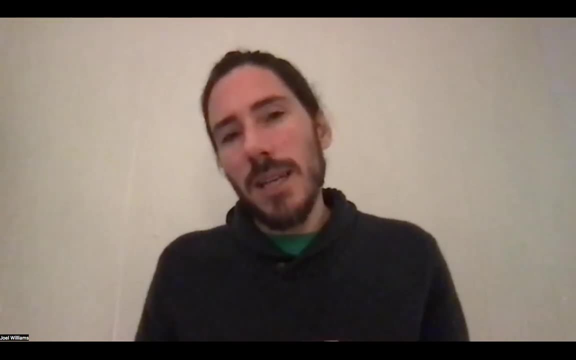 for example, to kind of spray some of those organisms out again with molasses or with the food source, to kind of feed them. um is is also a good idea. so yeah, i would say it's just would suggest to me that you've got a little bit of a problem with the. 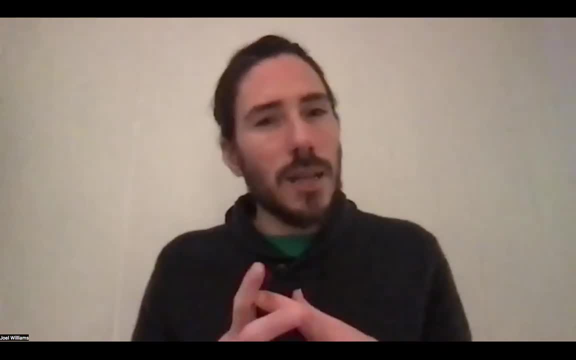 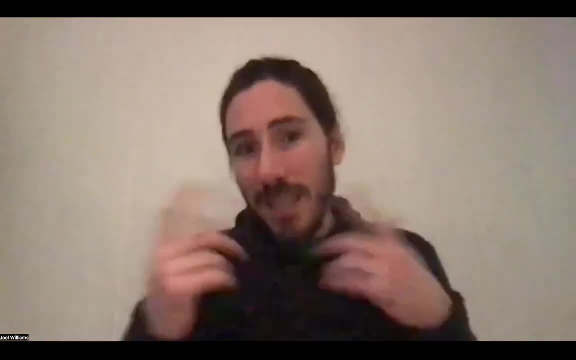 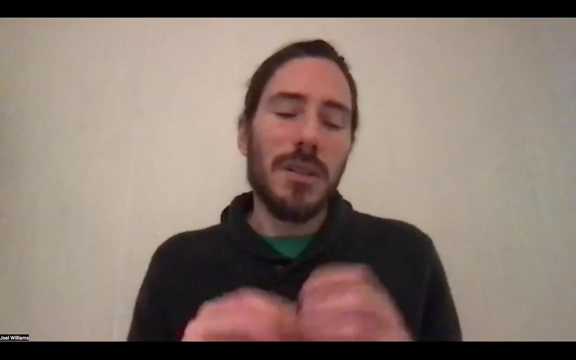 um, lack of biological activity. so just kind of prime priming the pump a little there and then beyond that, more longer term, i would look at increasing your plant species diversity. so we have i touched on just a few examples there, but we have pretty good evidence that the more 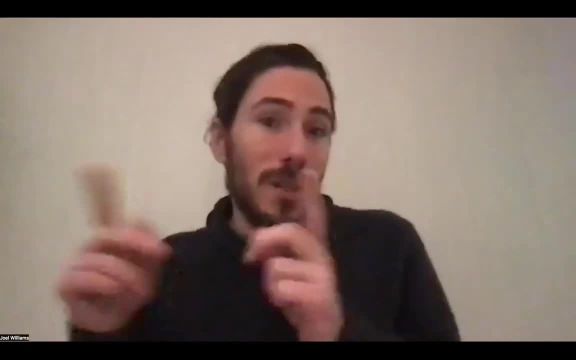 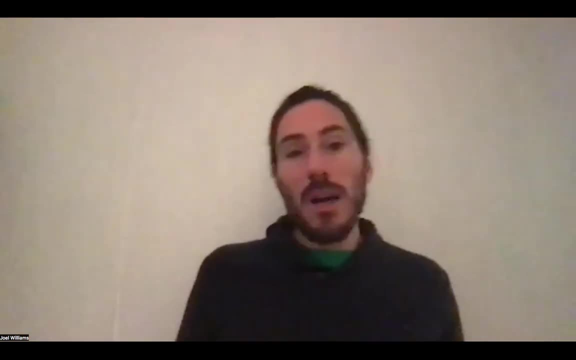 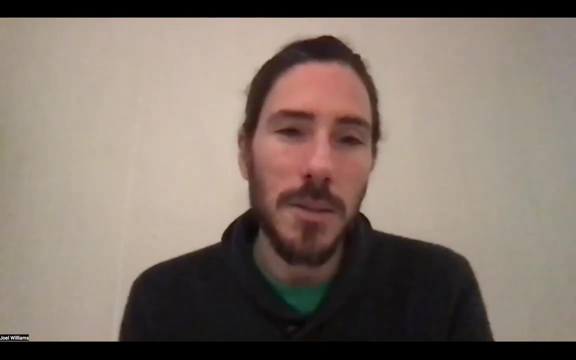 plant species diversity that you have. not only is that good for soil carbon, as i touched on, but it's also good for soil fungi, for many of the microbes, for good biological activity. so so, yeah, i would say that try longer term, try and increase your, uh, your plant species diversity. 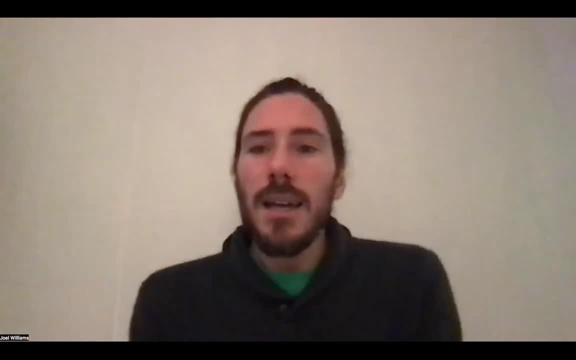 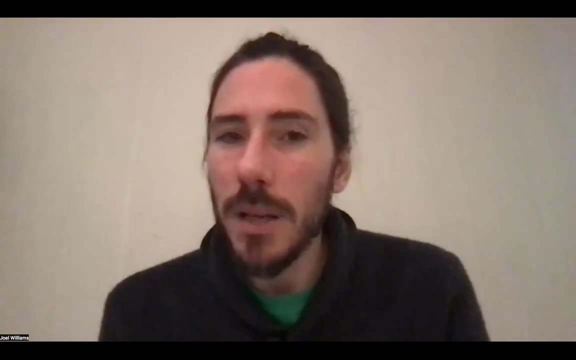 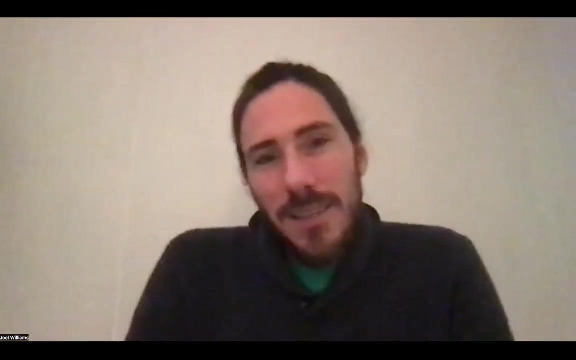 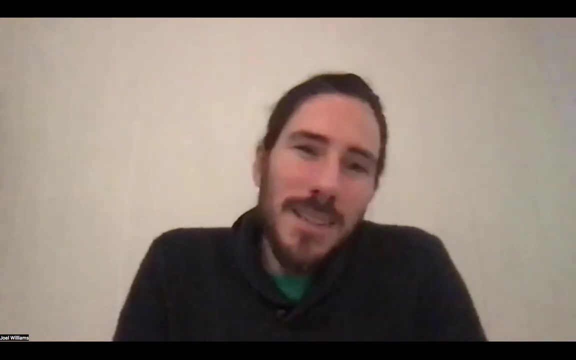 and uh. another question from michael. here it says: do symptom weeds such as thistles penetrate soils at higher rates than 300 psi? yeah, and this is a good question too, isn't it? this whole idea of weeds as indicators, i think, is a very interesting one, and you know, i think there's a mixed bag of examples out there. i think there's some. 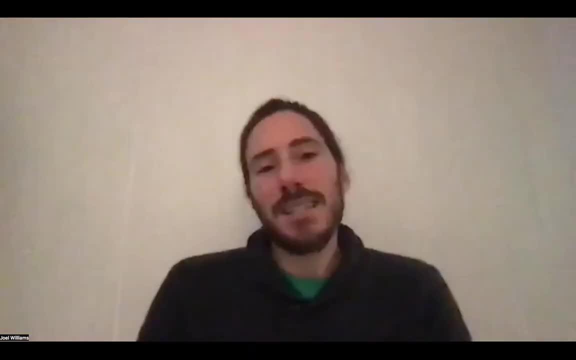 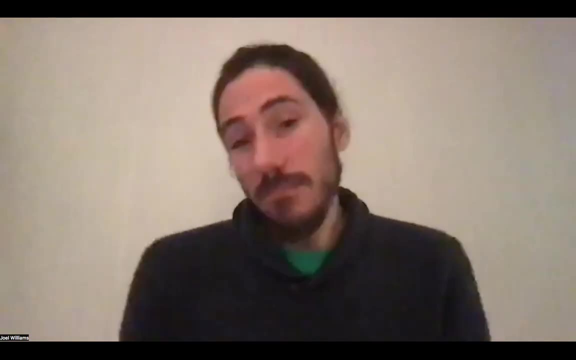 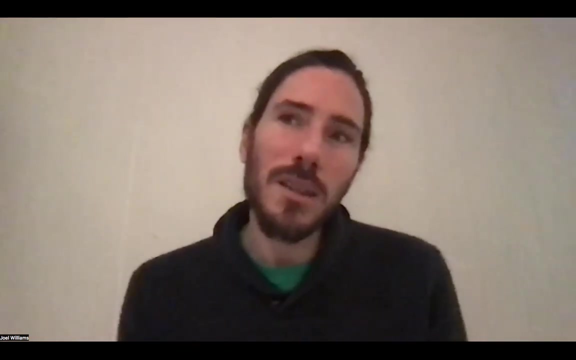 anecdotal type examples that are hard to say, maybe maybe not have relevance, but i think more broadly, the idea that weeds are indicators, i i agree. i sign up to this idea. i think it's true of all plant communities all around the world. they all grow where they can. they all grow where they. 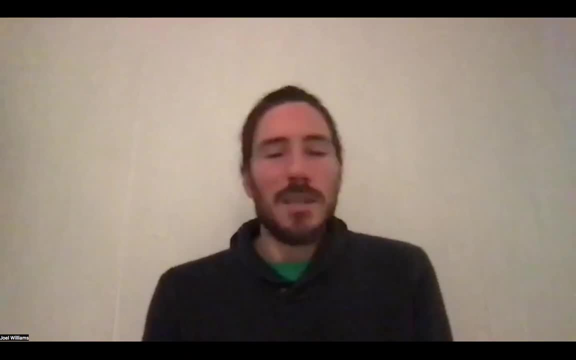 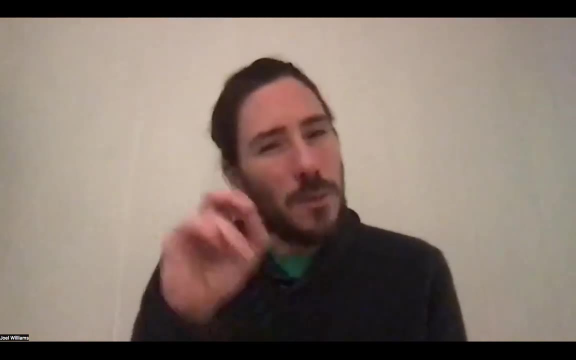 can thrive and um. so we see this already with things like this, and i think it's a good idea to do a lot of more, just to sort of back up the idea, the idea of doing voyages and all the different gitara things, i don't know, a fox trial barley. 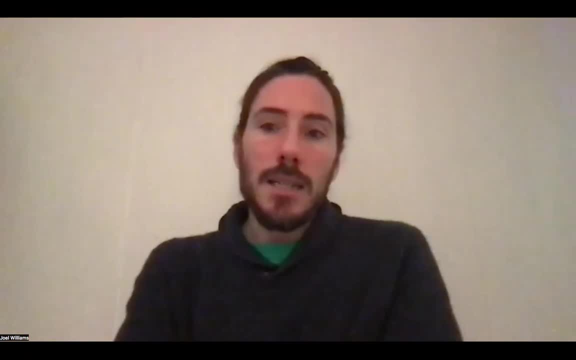 you know, growing in the salty areas, in the sloughs and things you know, plants were specifically seen to accumulate in certain areas. so so, yeah, i, i take on board the general notion that weeds are indicators. i think that's absolutely valid and um and so yeah, i, i agree, i think thistles, thessals, flour. 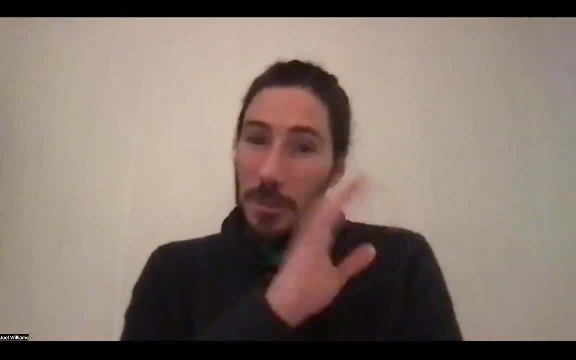 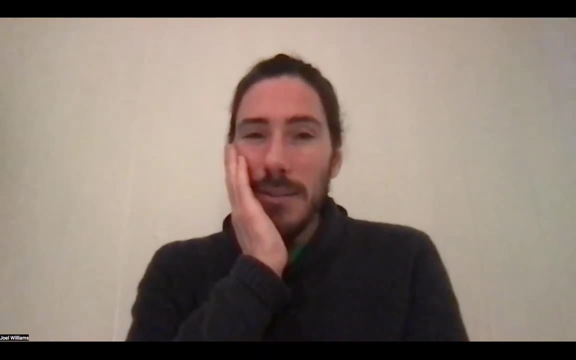 of compaction um thistles dejaiad spending money 1,000 scheintome theses. you're pretty much right at that limit where, generally it's considered, the plant roots don't penetrate so well. so you're kind of right at that cutoff. but i think when you're choosing examples 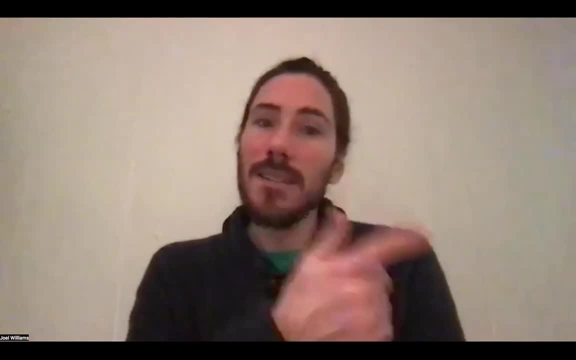 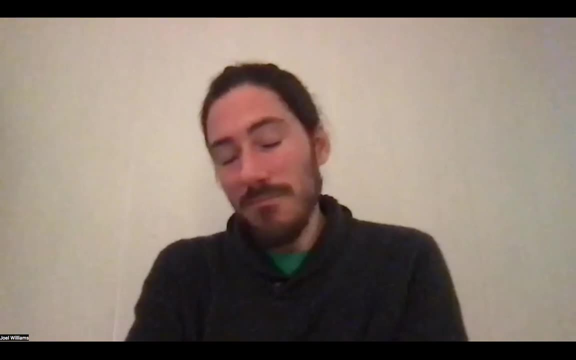 like thistles or like weeds that are clearly doing some element of soil repair or fixing the soil, that, um, usually they have specialized strategies to to do this and um, uh, yeah, i, i, so, yeah, i, i think that they're. if you've got a lot of thistles, it is an indication of compaction, that's for sure. 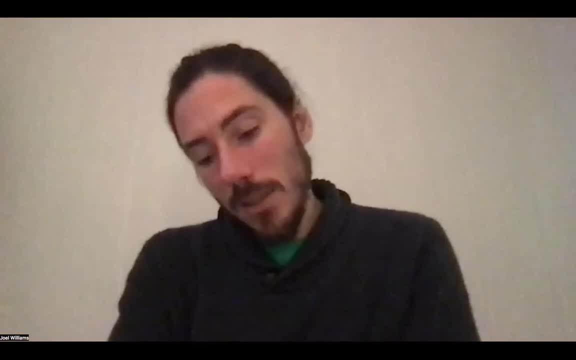 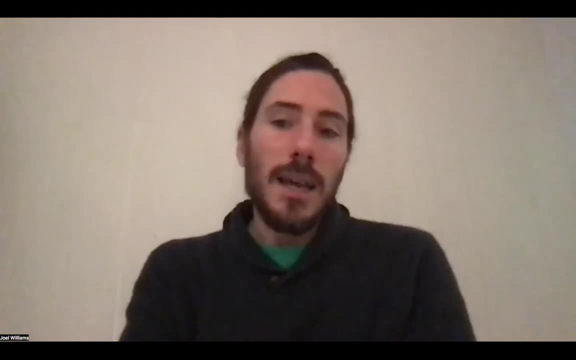 that's why they're growing there and um, uh, and so that would suggest to me that you need more deeper rooting plants- tap roots, fibrous deeper roots- and, um, you know, i would go and dig up some of those thistles. i was on a pasture farm in the uk and we would. this is maybe because this is. 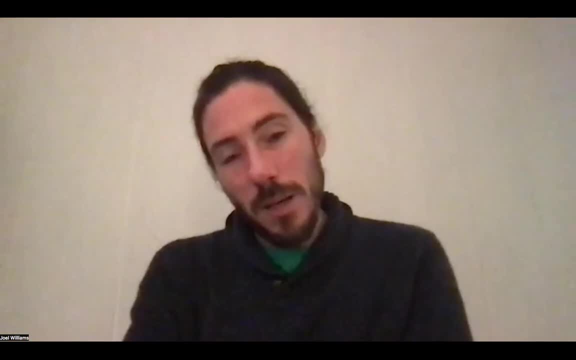 pre-covid a couple of years ago. but you know, we were just going through some pastures having a dig in the soil, digging some kind of some quick spades and having a look at the soil structure and that kind of thing and and you know, yeah, it was pretty a bit tight on the soil, not great root. 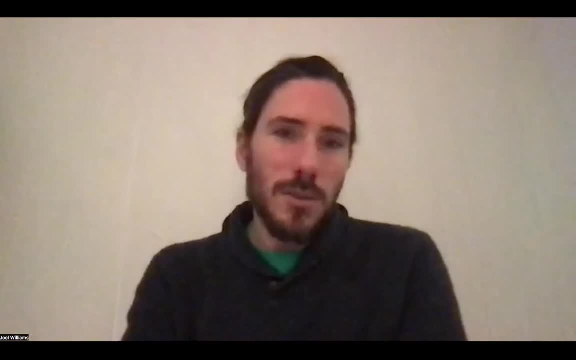 growth and, uh, there was a few- this quite a few thistles, not hugely heavy, but there was some thistles in the field and, um, i said, yeah, let's go dig some of the thistle and and with the farmer, and, yeah, as we dug up that thistle, of course the, the roots just looked absolutely fantastic. it was. 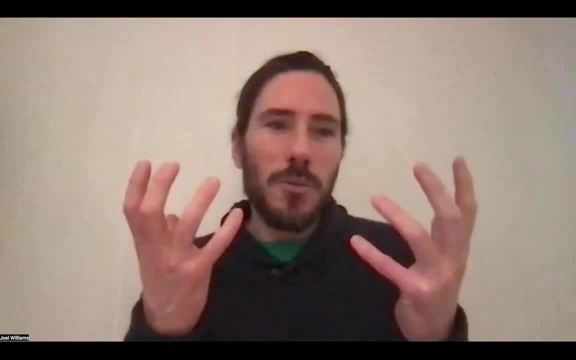 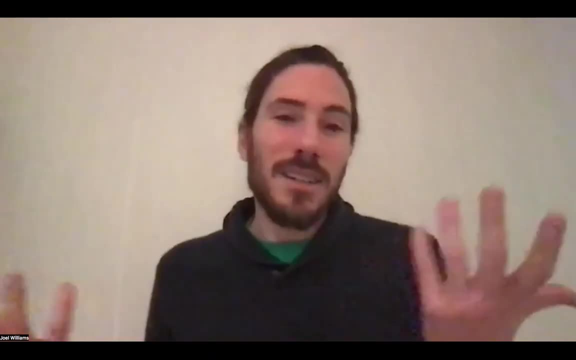 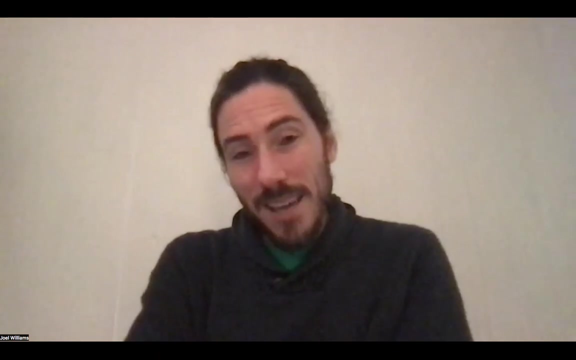 absolutely full of earthworms and the smell of soil was fantastic. the root, the soil looked really well structured, but literally just right next door you would dig the grass, pasture and and so just look completely different. um, so, so yeah, i i think that weeds have specialized skills. that's why they're, that's why they're growing where they do. 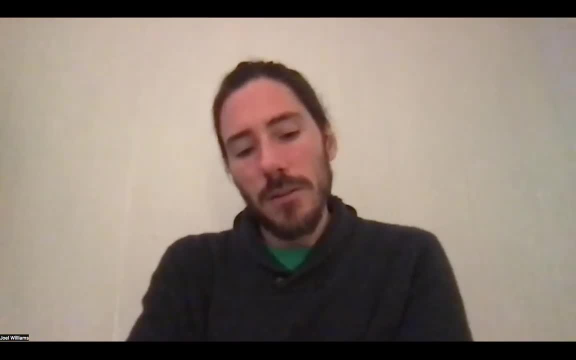 and why they can be problematic, and we should definitely fine-tune our senses to to kind of read what they're trying to tell us. but, um, but whether or not exactly plants will penetrate higher than that, i think it's a bit context dependent a bit there. but um, i think in the 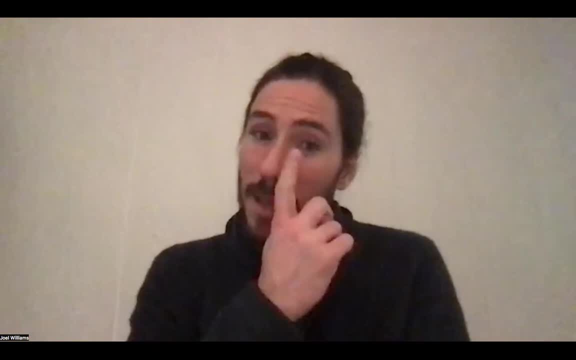 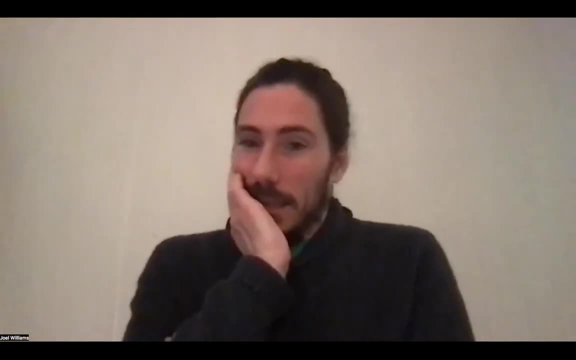 example of thistles, it's it's probably telling you that, that they can and they're signaling that the compaction is an issue. so, uh, okay, question from jerry here says: uh, grazing pigs and concerned about compaction, they return every 15 years. alfalfa, timothy plantain radish. 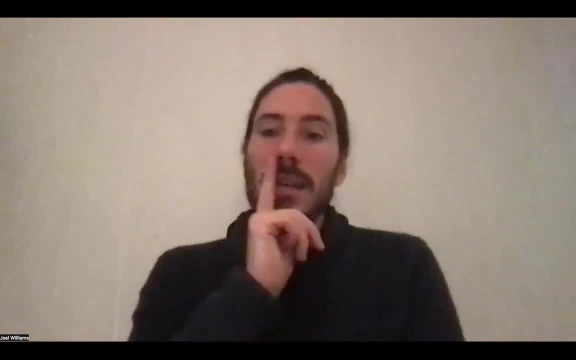 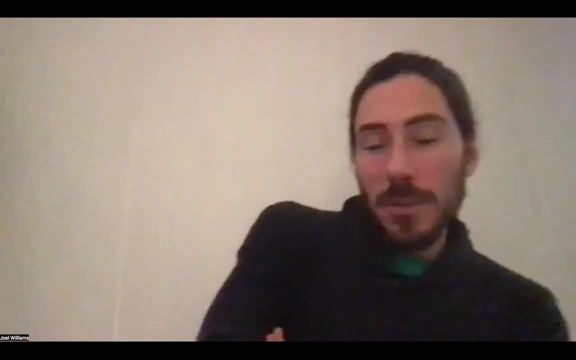 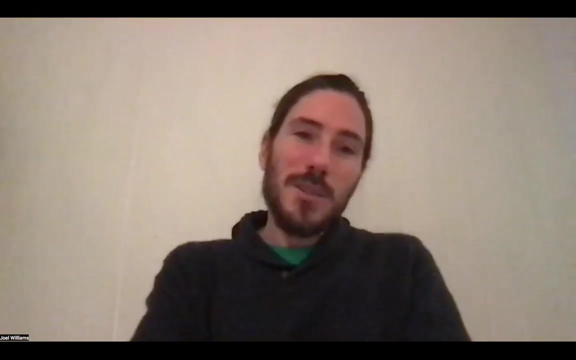 for the springs, for the springs seeding, yeah, you know. yeah, it's a good question too, isn't it? it's? of course i know pigs are pretty disruptive, and of course they are, but again, i don't know animals. they do this in nature, don't they? um same with this whole point about trampling and 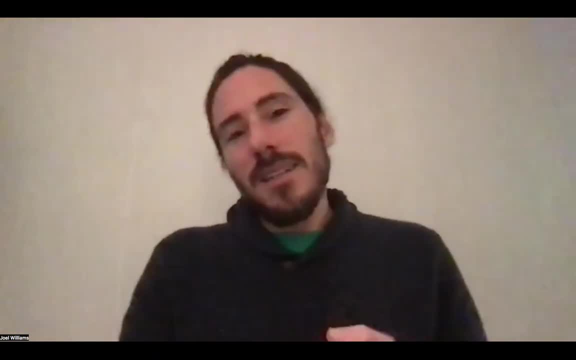 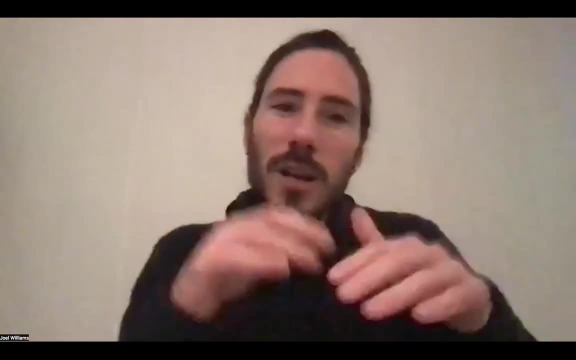 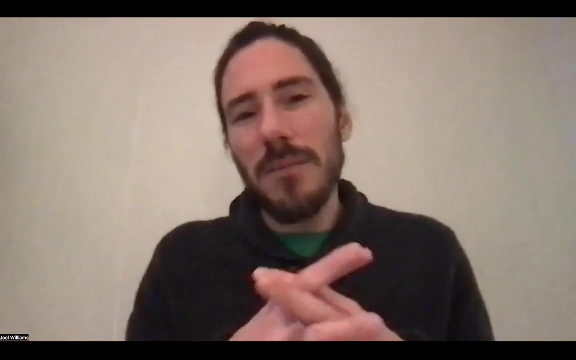 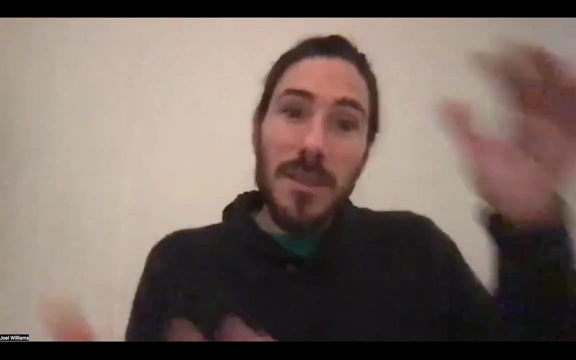 surface compaction from livestock and hooves- like of course too much of it- is definitely bad, but a little bit, and a little bit of integration of st지bbles and residues into the soil through that, through that trampling, and its not so intensive in inversion but it's, it's light working from. 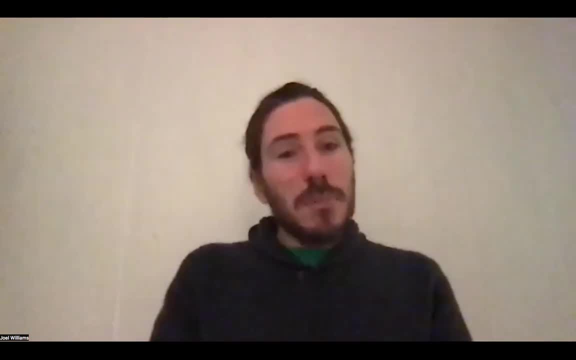 the surface light incorporation. it's very beneficial. you know, a little bit of that surface disturbance can just help to stimulate micro activity, to stimulate residue breakdown, and i think that's something we all have to look at as well. so i think it's it's important that we really decide how we do it. we all have to do it, but i think that's actually 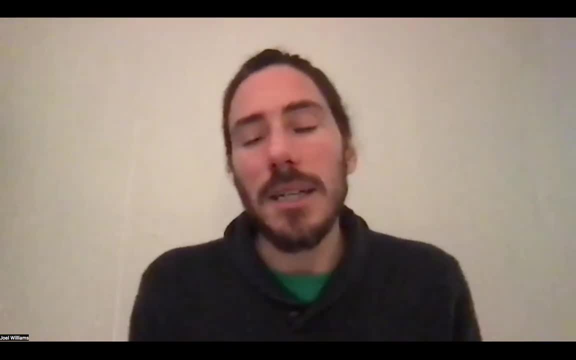 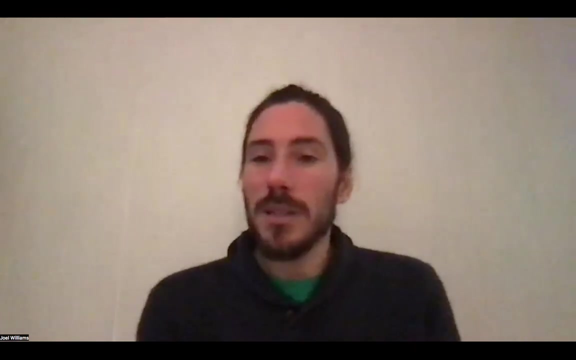 residue breakdown. to the question also earlier: um, having a little bit of that light incorporation, better soil contact with the residues- also another strategy to to increase that residue breakdown. so so yeah, of course pigs are extremely disruptive in that sense, but um, it is a, it is a natural. 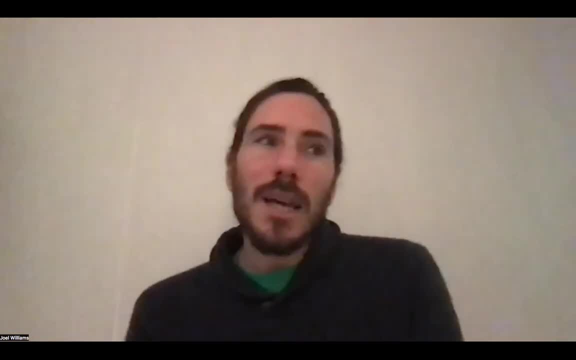 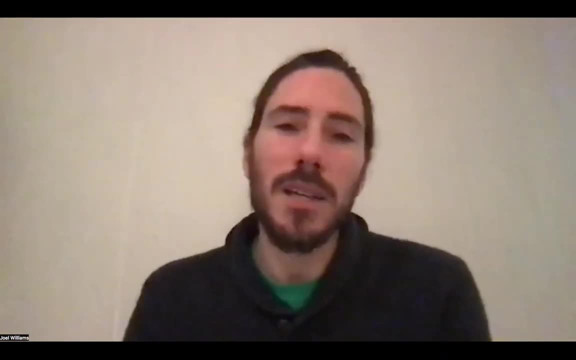 process, just like animals kind of do, and i think that, um, you know, they're a great way to kind of plow the soil and if, if you're at that point where you need them, breaking a rotation and moving from a grass into a cropping situation, you need to terminate that grass. um, you know. 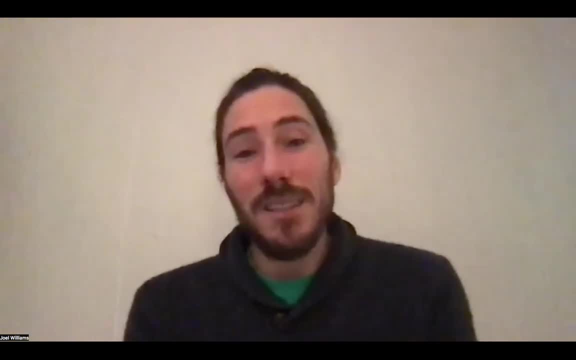 pigs i'm sure have a role to play, and okay, if you're not returning for every 15 years- i mean that is a long time for recovery. so that sounds excellent for me. to me, um, i think you're giving the soil plenty of time to recover and you've listed off the right species to help you do that with deep roots: alfalfa. i mentioned timothy, i mentioned plantain. i totally agree, you know. so i think that you're giving plenty of time for root recovery, for root growth, for restructuring of that soil. i'm definitely much more problem if you were to come. 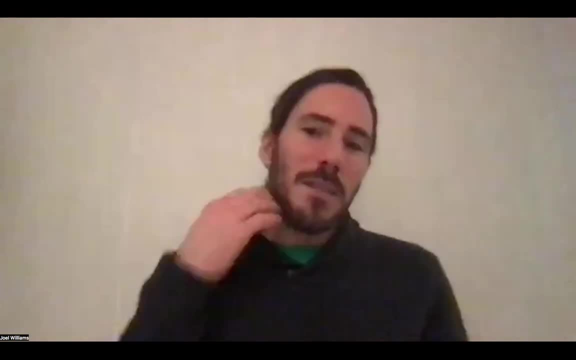 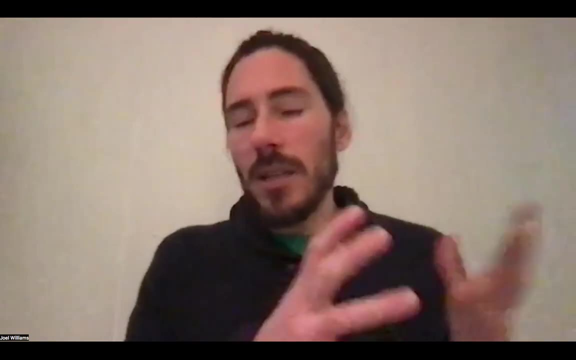 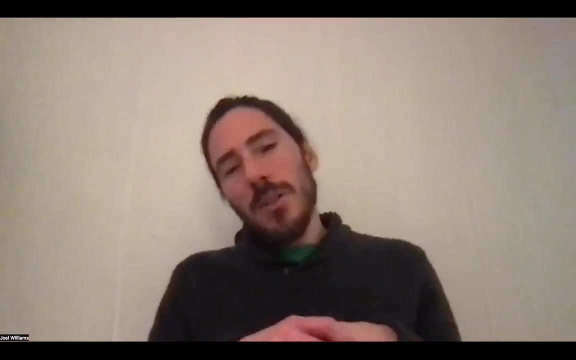 back, you know, within a few years and boom, do it all again. but i think that you're giving yourself more than enough time um to address that compaction that they, that that they will cause during that time and um, and i think that's okay to some extent. you know that's the part of the process of 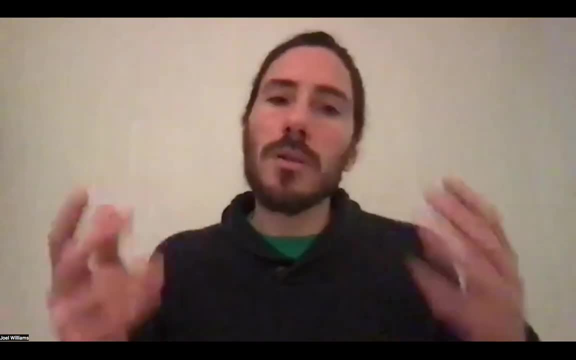 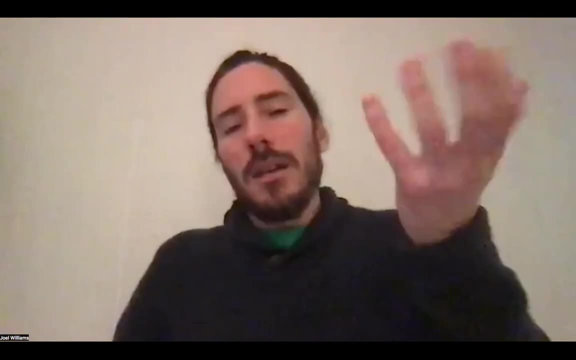 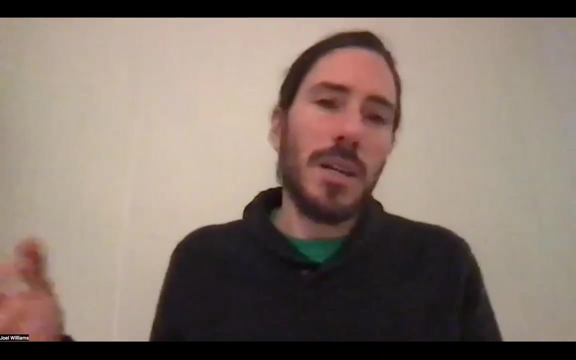 for example, building fertility in the soil or building organic matter. you, you want a phase where you're building fertility, building soil, organic matter, and then you want a phase in the rotation where you're drawing down from the bank, where you're harvesting that fertility. you're using it for production. you're using it, therefore, to make money to run the to the. 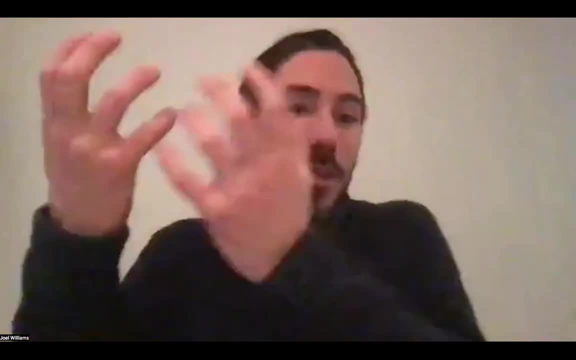 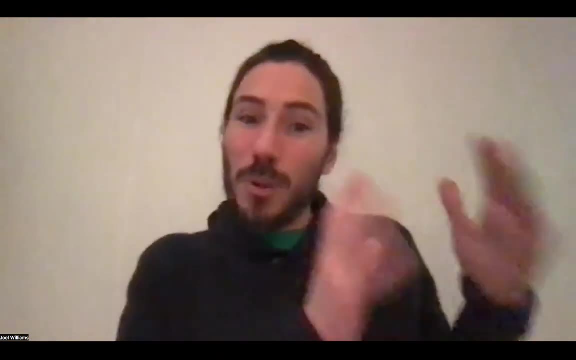 plumbing side of the business. you've got to build and you've got to use it's. it's not all about sequestering carbon building, carbon building cut like, it's not all about that. that's important, of course, but you've also got to use drawback on the fertility that you build as well. so i think that over a 15 year period. i i would imagine, unless you tell me that you're still seeing heavy signs of compaction, um along that 15 year gradient. um, i would think that that amount of time is is enough for soil recovery and and and soil rebuilding, and then that's just how it is. 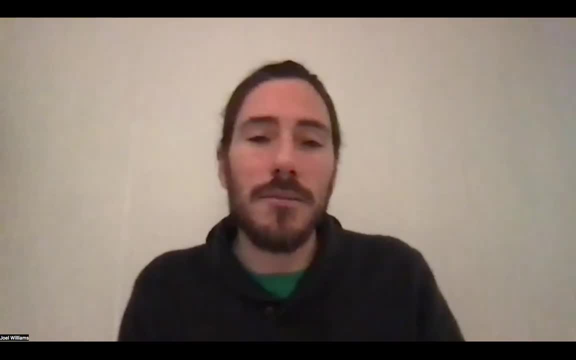 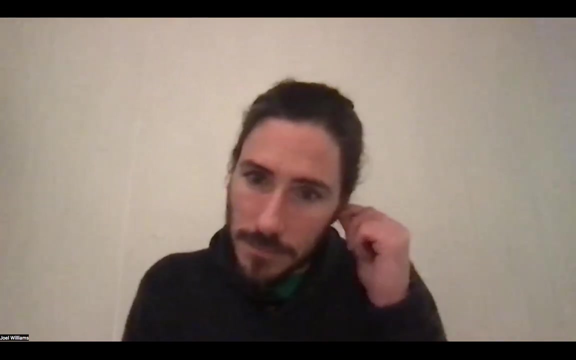 you're running a farm, you're running a business. you've got to bring those animals back for for the economic side of it, and as long as you didn't do that so quickly and you've built soil in between, then then i think that's okay awesome. thanks so much, Joel. well, thanks everybody.